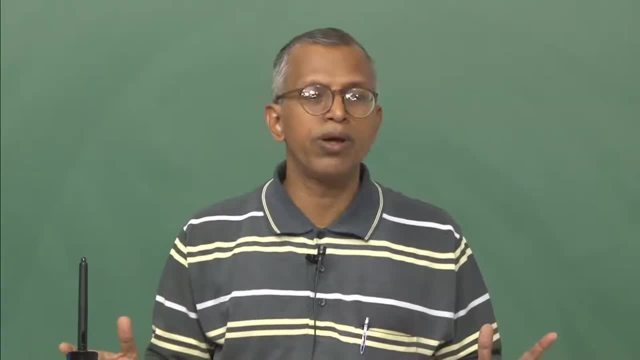 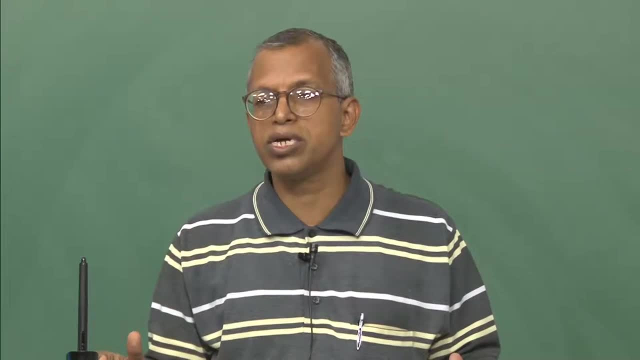 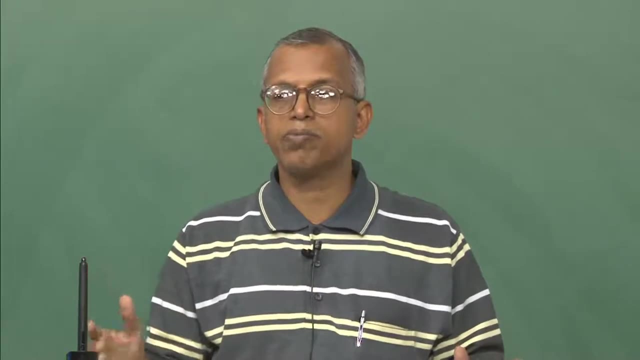 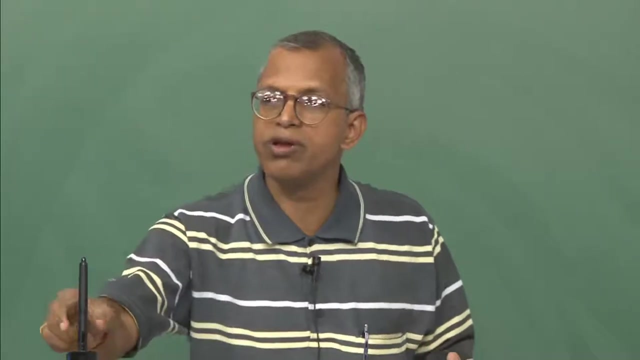 We did not really bother about structure of the flame. we assume there is some heat release rate and then we, you know, use this conservation of mass momentum and energy equation derived the expression for what you call various properties like pressure, density, other things. But today we will be looking at one dimensional premix flame. and if you look at one dimensional 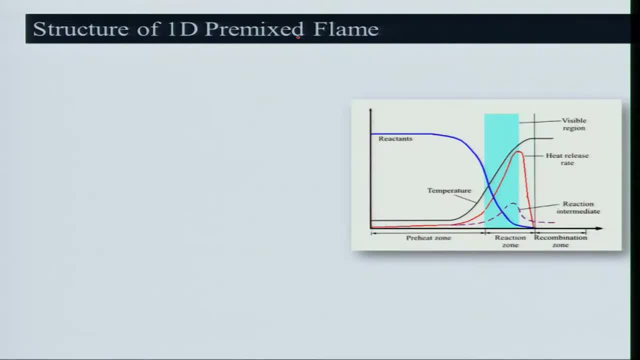 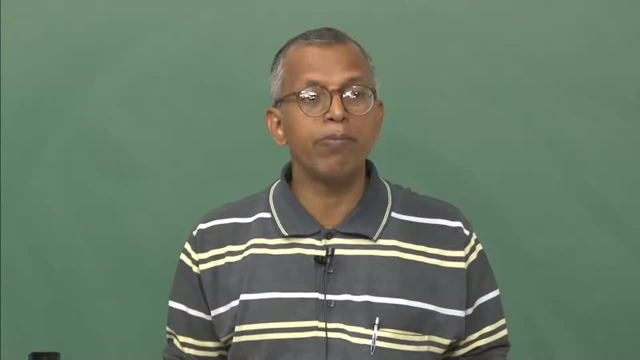 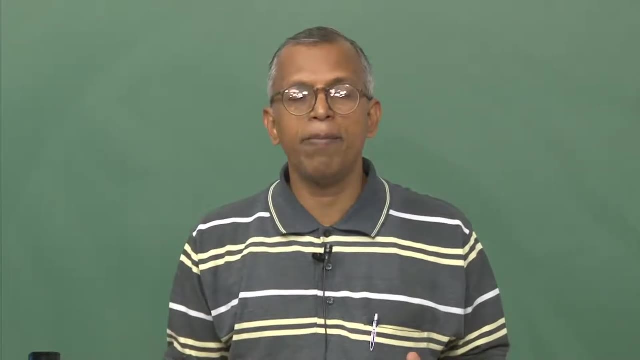 flame can be obtained in the laboratory, but in natural it is quite difficult to have that one dimensional flame. Of course, if you look at the premix flame is basically a manmade flame. you can assume, as I told, that Bunshan had, you know, found out that flame. 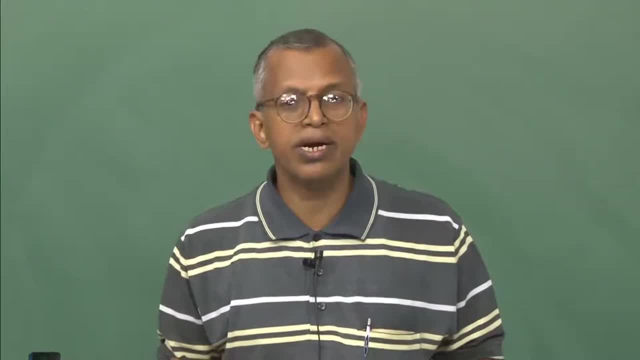 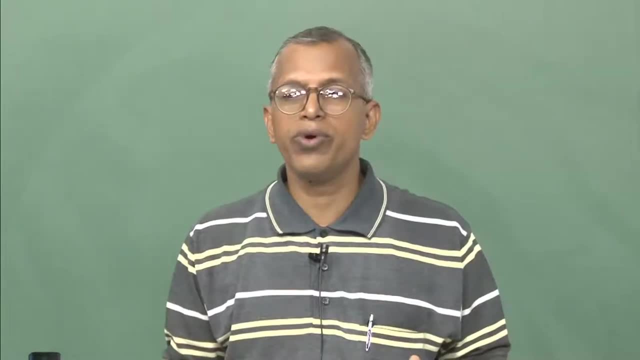 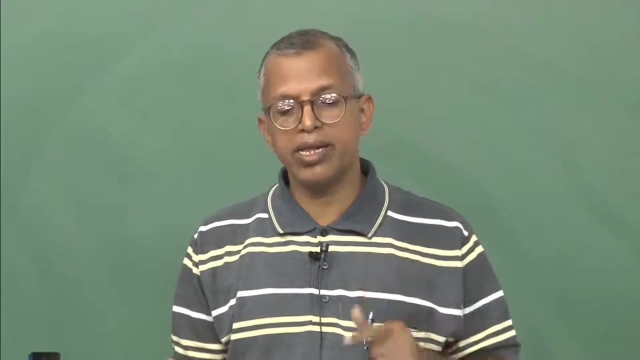 And of course one can assume, because you can stabilize in a burner and then one can assume it to be one dimensional. Therefore, similarly, in the, we can use one dimensional burner and then establish a flame which can assume to be one dimensional. keep in mind that here what we will be discussing is laminar one. 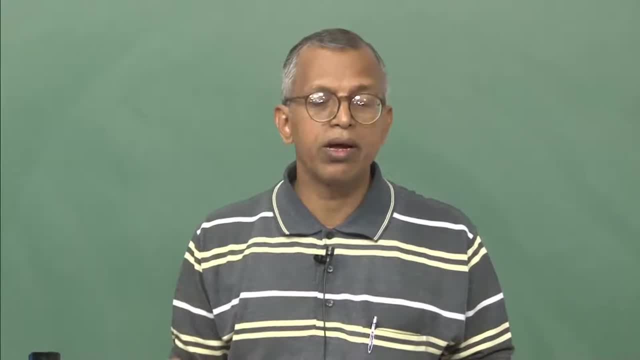 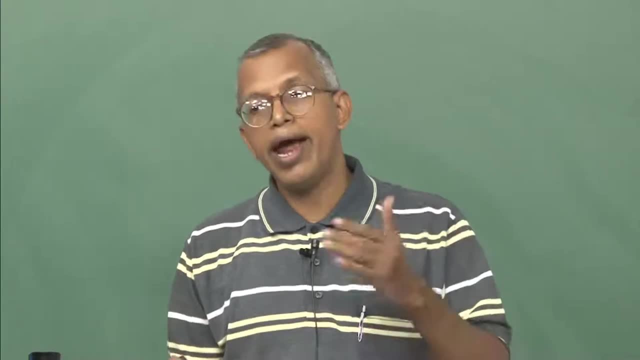 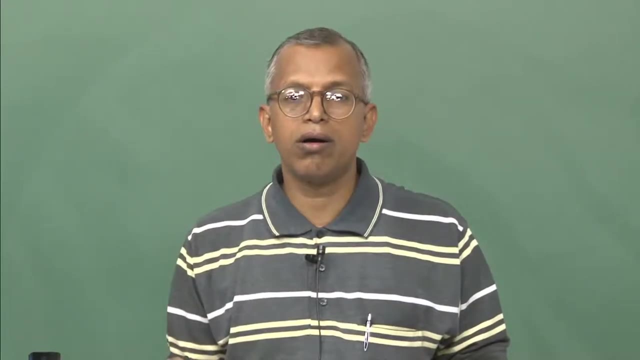 dimensional premix flame But in nature, most of the you know flame will be turbulent in nature And also in the practical situation it will be turbulent. So therefore, you know it is important to look at turbulent flame but, however, due to complexities and other things, 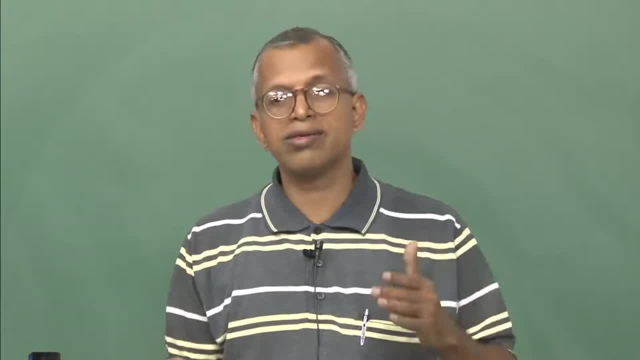 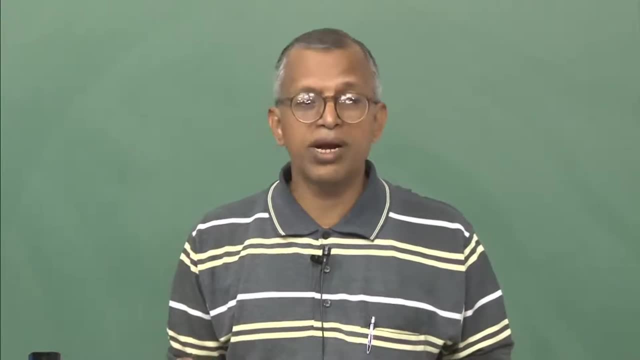 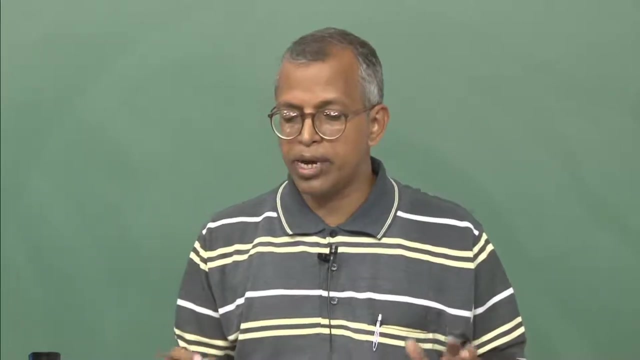 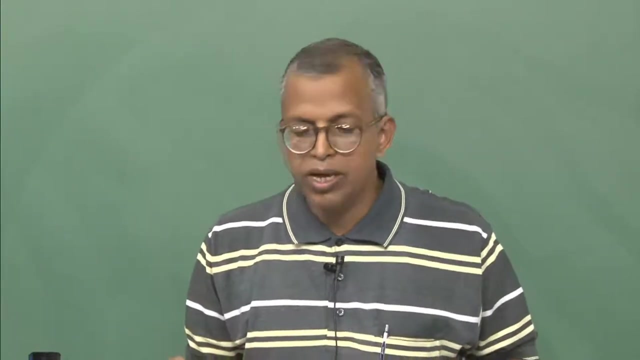 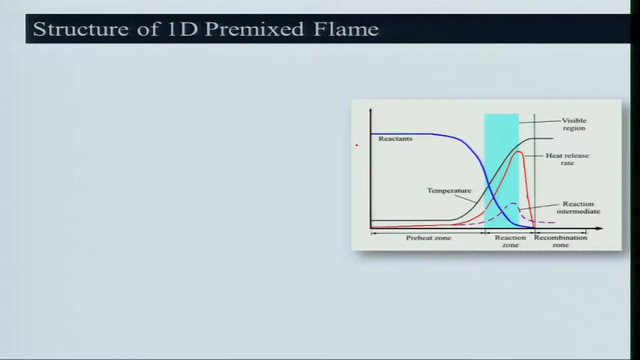 we would not be looking at because we can relate this laminar flame to the turbulent flame, particularly when we will be moving to the gas turbine combustors, Then I will be discussing or touching upon that turbulent premix flame. So if you look at what you observe, whatever you know from here, I have plotted here in. 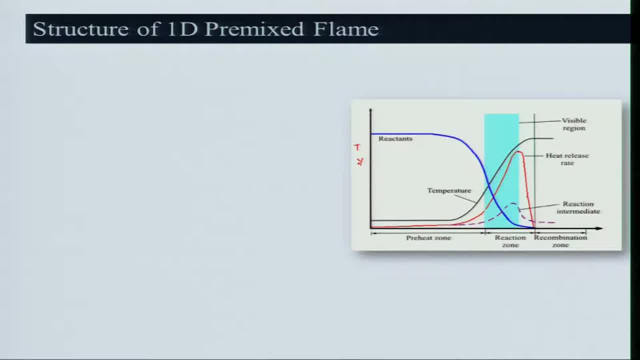 this vertical axis, temperature, mass fraction of, you know, fuel and oxidizer. If you look at this is basically mass fraction of the reactant. you know reactant can be fuel, can be oxidizer And of course there will be a part, and if you see this, that it is, you know, decreasing. 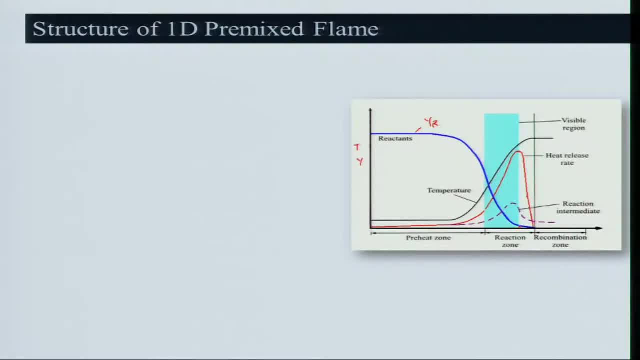 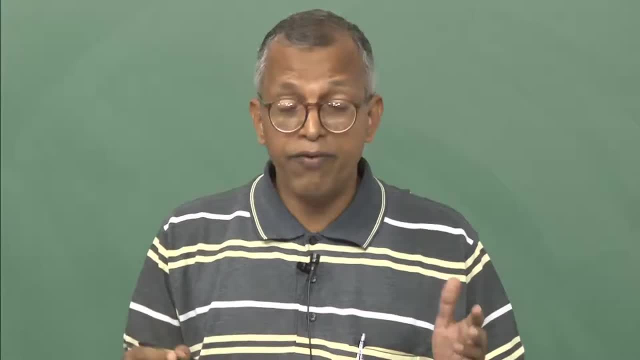 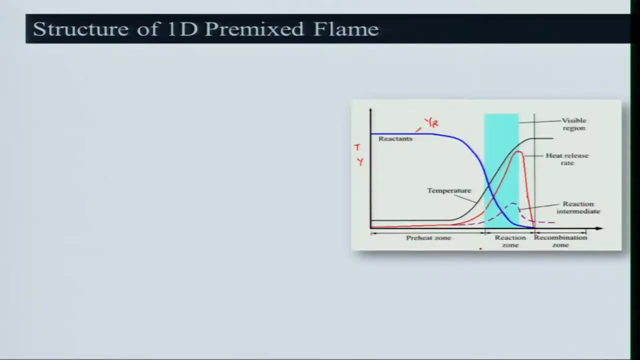 that means it is consuming this mass fraction of the fuel. And also you can have a similar plot for the or the variation for the mass fraction of oxidizer. it need not to be same but it will be similar. And if you look at what you can observe here, that in these zones 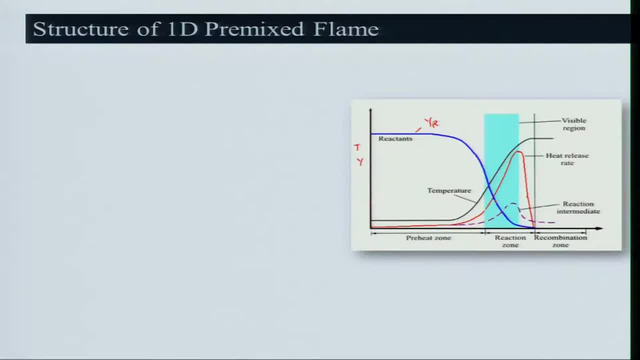 the gradient is very high, and not only for the mass fraction of the reactant, but also for the temperature. Temperature is being shown here right and there is a lot of heat being released in this zone if you look at this red one: heat being released, peak value. 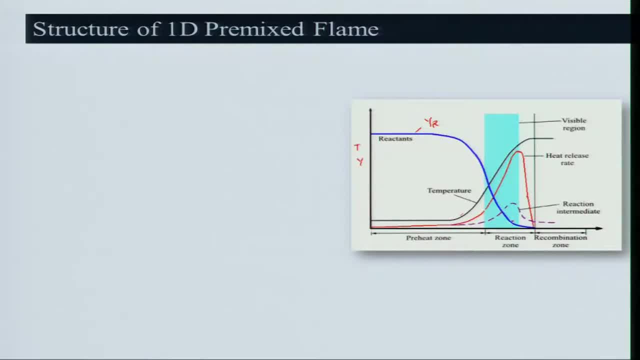 and then it receded towards that. And of course there will be some intermediate reaction will be occurring. you know reactants and the reaction will be occurring and some of the reaction will be occurring. So this will be a load to theolina because some of 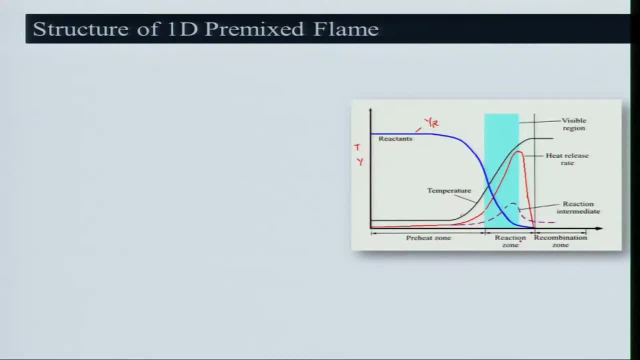 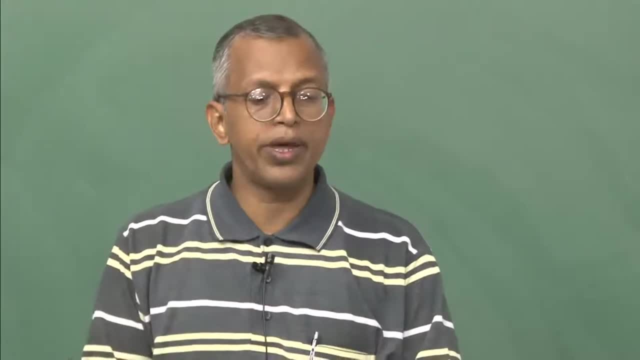 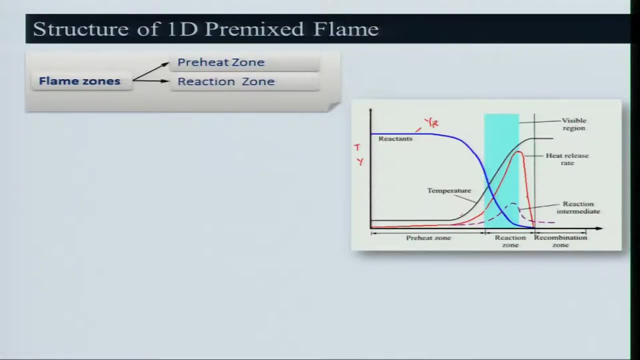 occurring in this region. So if you look at the flame can be broadly divided into three categories. that means flame in the sense, flame zone right. This zone can be broadly divided into preheat zone, reaction zone and recombination zone. What is really happening? 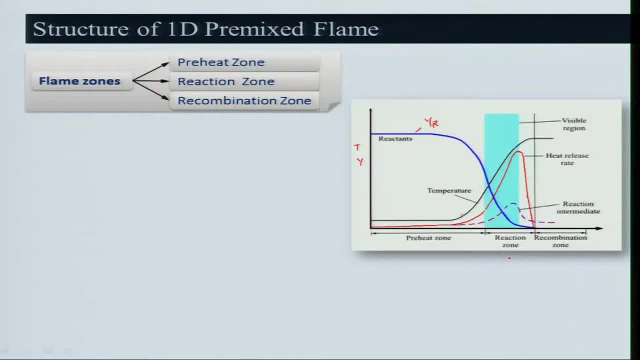 in this preheat zone. If you look at, temperature is not really going up, but a little bit, you know, slowly increasing in this zone. because why there is a negligible heat release. If you look at, heat release is very, very small in this domain alone, of course, with that, 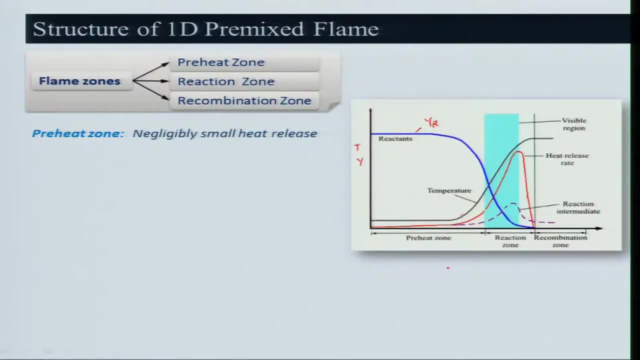 temperature also, you know, suits up So negligibly small heat release is occurring and certain chemical reaction does occur. Do take place in this zone, which I have not shown may be some of the, you know, like a space is like H O, 2 or H O or something will be occurring in this region because of temperature. 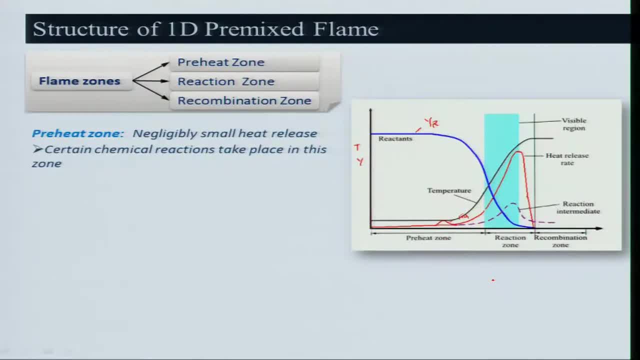 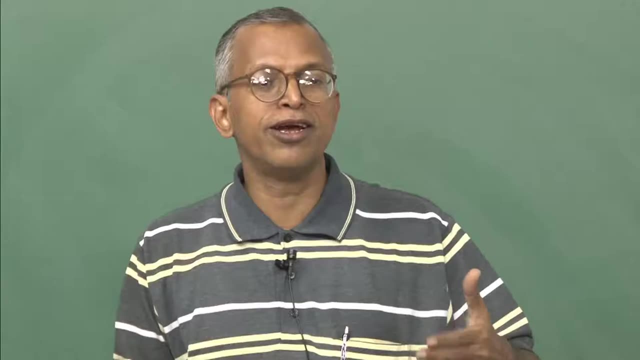 is being little bit shooting up, But however, you know like it is not that if I compare this preheat zone with the life of a human being, what it would be- nothing really is happening productively. So for flame, Flame is concerned, flame is basically what, where the exothermic reaction will be taking. 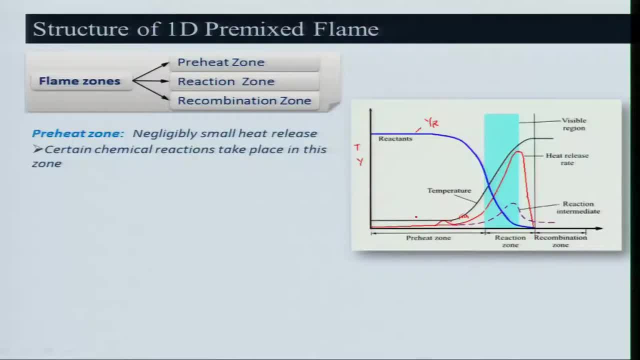 place The, if you look at overall in this zone, particularly overall reaction. whatever it will be occurring, it will be what you call net effect will be nullified, that neither exothermic nor endothermic temperature is remaining constant. but in this case there 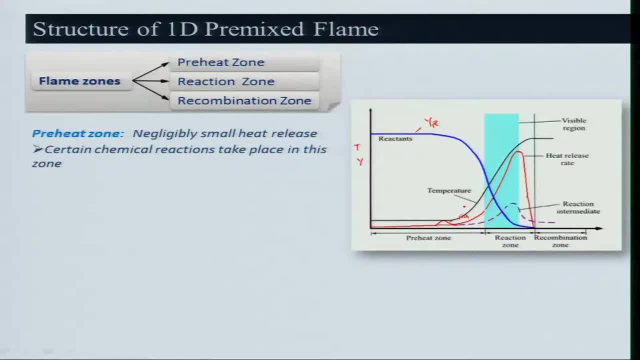 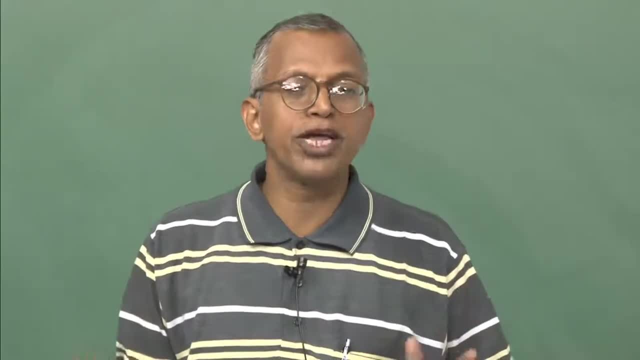 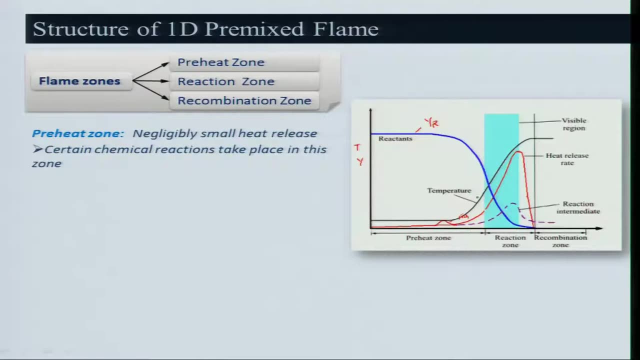 will be little bit increase. So this will be similar to your what you call student life, where you are being prepared to do a productive work During your adulthood, kind of things. So but whereas all this gradient- you know gradient- is occurring or the temperature, heat being released in the reaction zone, Of course. 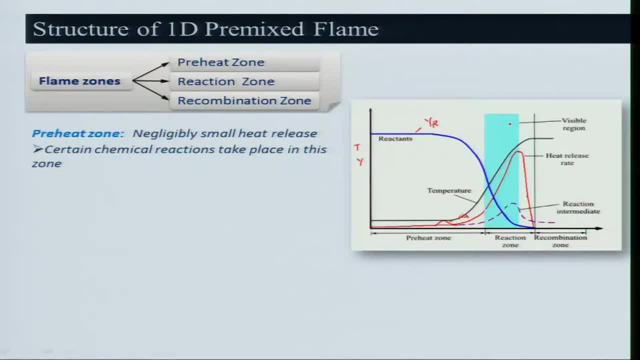 the zone. in this there will be several spaces which will be liberated, radicals, and that will be radiating, you know, various spectrum of the light which you can see, for example C A star, O, H, and then C 2 star and other things. 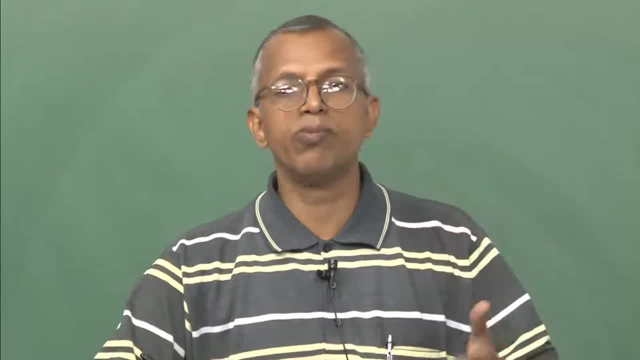 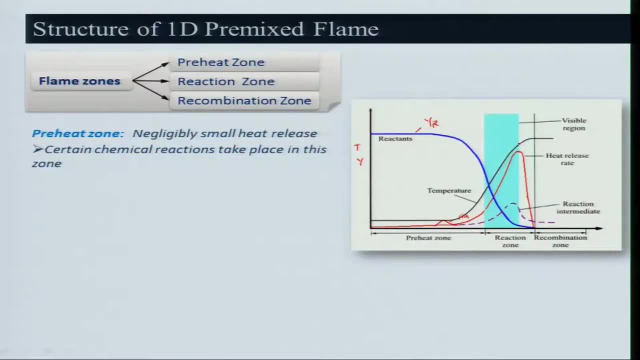 I discuss those things. you know, C A star will give a blue and then suit if it is the yellow, and then some purple color. all those things will be coming. So you will see that and keep in mind. this is the reaction zone, which is very thin as compared to the preheat zone. 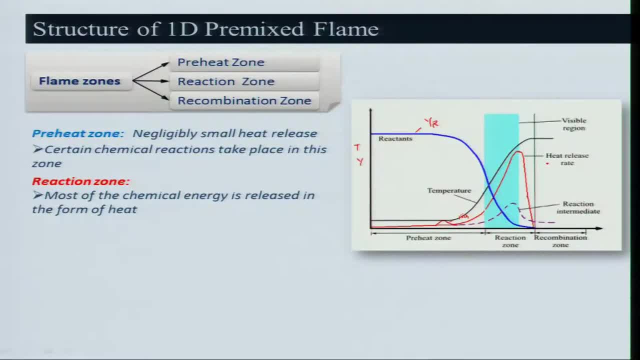 And in the, if you look at that means in the reaction zone. most of the chemical energy is released in the form of heat in the reaction zone and decomposition, of course, will take place. And these decomposition really not take place in reaction zone, it takes place in the beginning. 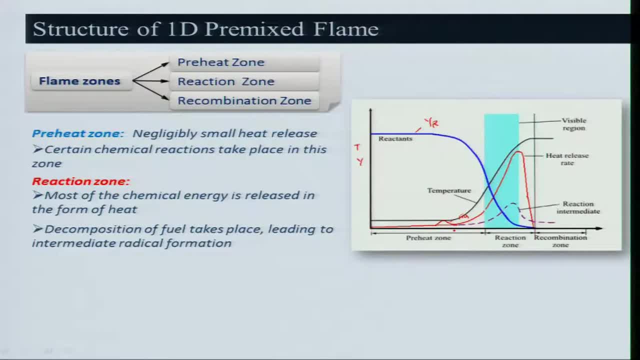 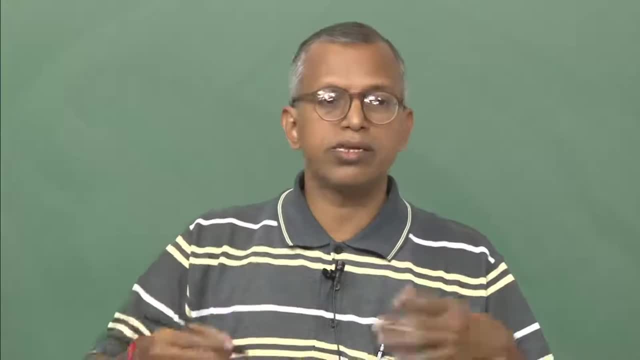 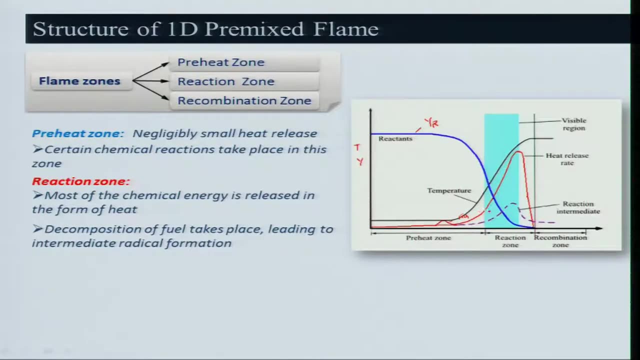 of the reaction zone or just before the reaction zone, because there will be paralysis product or the decomposition of the fuel, Like, for example, propane. propane will be converted into methane, some other things, and then goes on like that. So that will be creating some radicals, you know to be what to call be consumed in these. 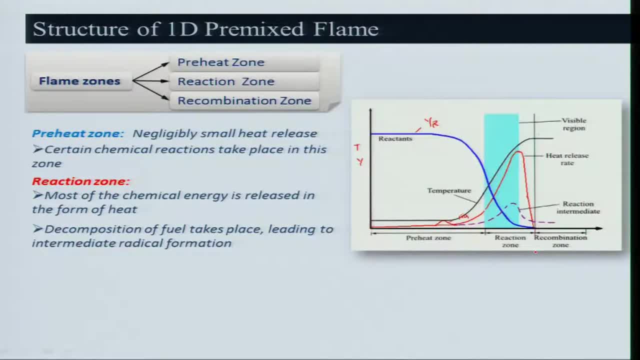 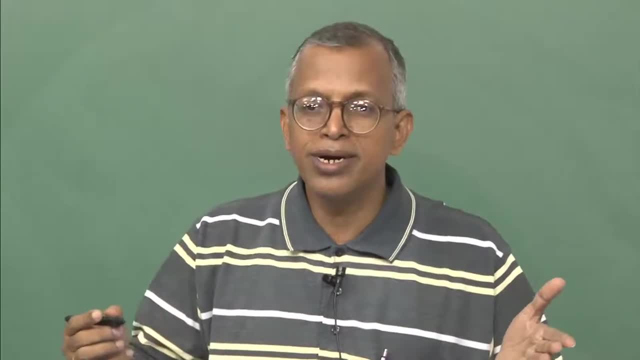 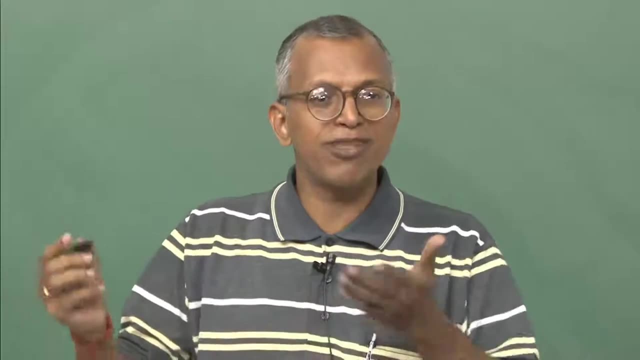 reaction zones. And that is very important because whenever I see a flame I always feel it is a life like life is getting. you know flame is getting burnt like fuel is being getting burnt, So also in life you getting burnt your time. you know time is receded as you go on And you 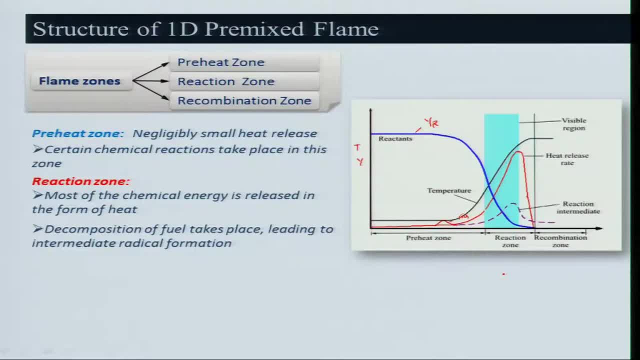 get prepared to contribute for the life, which is not being done through education nowadays. but in principle it should be like a flame: it prepare the spaces to be consumed in the reaction zone and then it will release heat and also the light you know, So that it will. 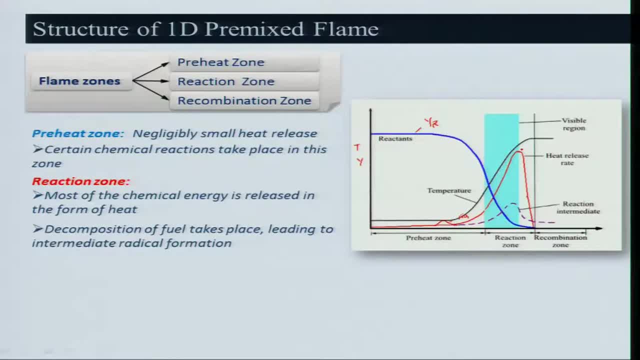 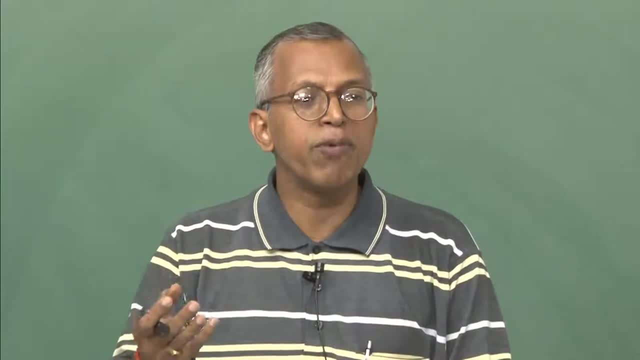 be people can take help. So reaction zone is very important, So also the productive life of a human being. one should not be really only worried about his food, he should worry about what he can contribute for the others. So reaction zone, as I told, it is very thin. 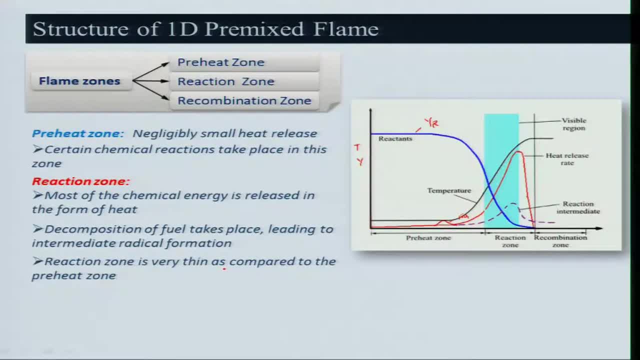 as compared to the preheat zone And keep in mind that this is the very critical part. So, for analysis is concerned, and because the gradient is very high here, right, and temperature gradient and concentration case and high, as I told you, And recombination zone, this is this zone particularly, you know, is basically 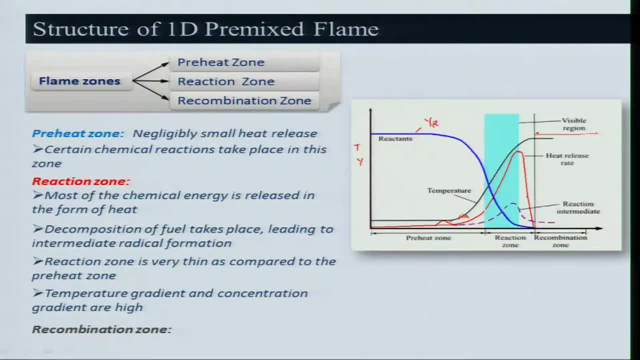 the recombination zone where I have shown here, temperature should be almost flat. there is no change in the temperature, Along with the x direction. if I say this is x direction, then you know there is no change. but in real situation, particularly for a hydrocarbon, you know this thing- there will be some recombination. 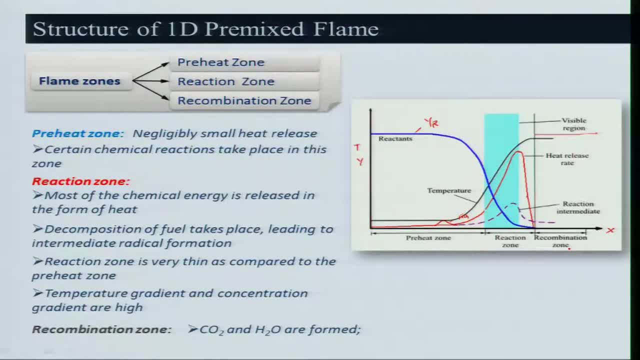 like carbon, you know, dioxide and water will be formed And some amount of heat being released, particularly for hydrocarbon. as a result, the temperature profile will be increasing towards the asymptotic value, which I have not shown deliberately. So you know, I want to simplify and then analyze it right. So if you look at you summarize: 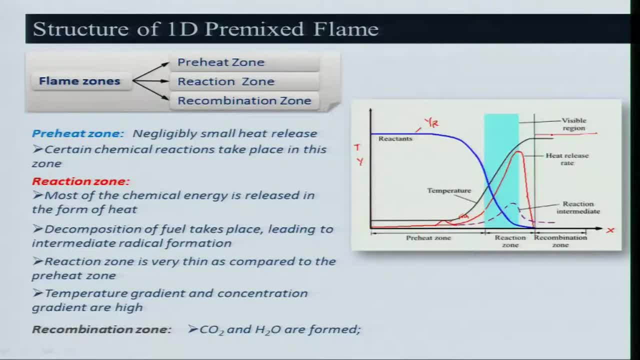 the flame zone can be divided into three. you know, one is preheat zone, reaction zone and recombination zone. And you should be careful about this, because what will be doing? we are not bother about this recombination zone when we will be analyzing and this one dimensional? 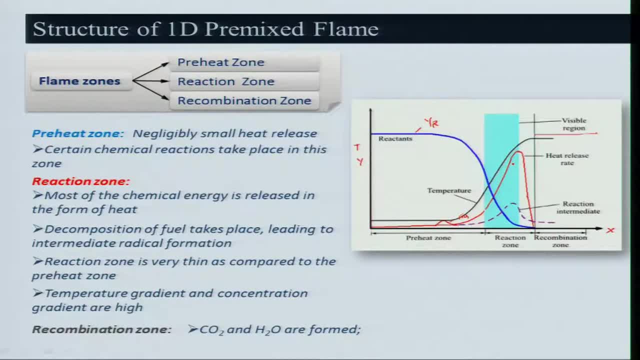 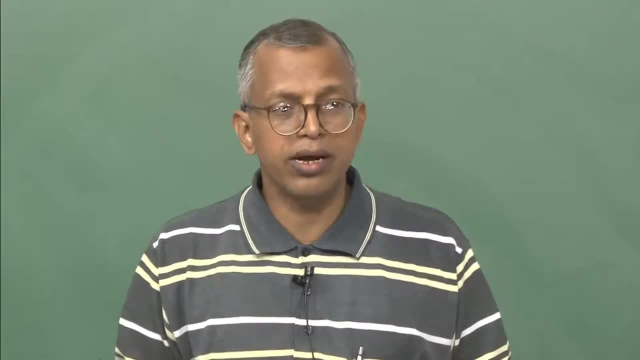 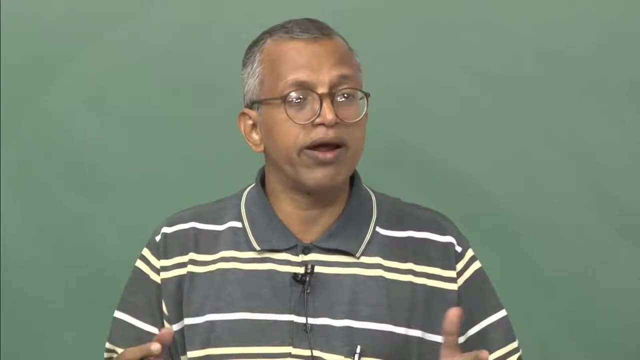 flame will be bother about preheat zone and reaction zone. What is really happening here has to look at it like if you look at the various processes are occurring, like if I look at the thermal side, you know, then there is a conduction, there will be convection there. 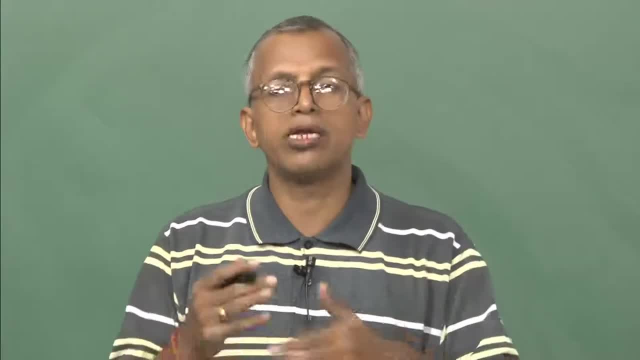 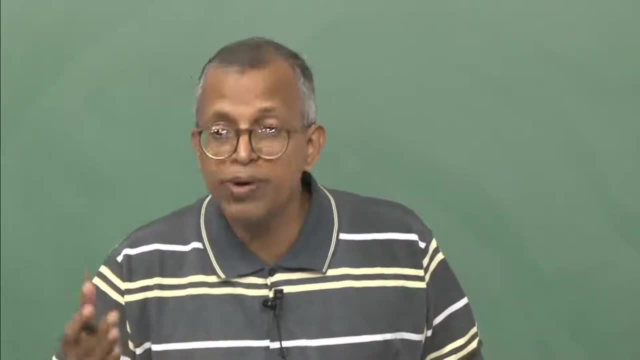 will be also radiation, you know heat transfer will be taking place and some chemical reaction will be taking place and it will be preparing the- you know- fuel and oxidizer to be burnt in the reaction zone. So of course in the recombination, as I told, 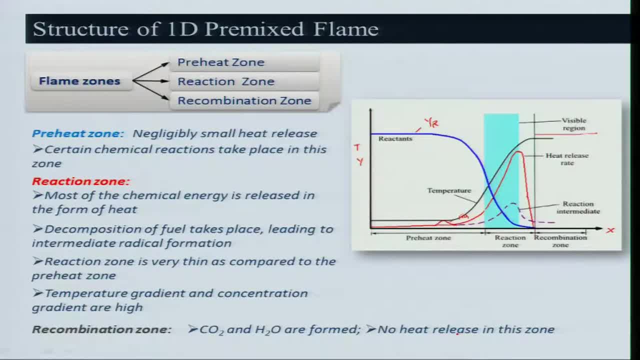 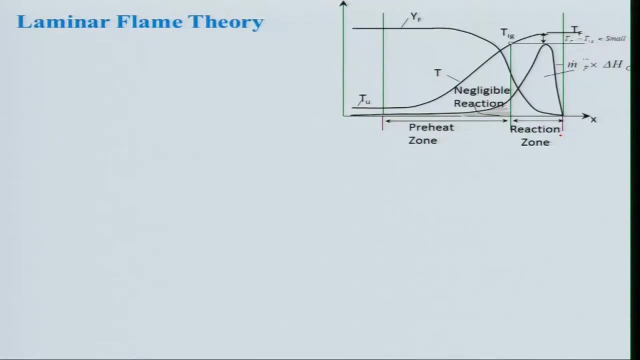 you, the no heat release in this zone is being occurred for our case, but in that but whatever, the heat release being occurred in real situation is very negligible, small as compared to the in the reaction zone. For the practical analysis purposes which we will be doing, keep in mind, 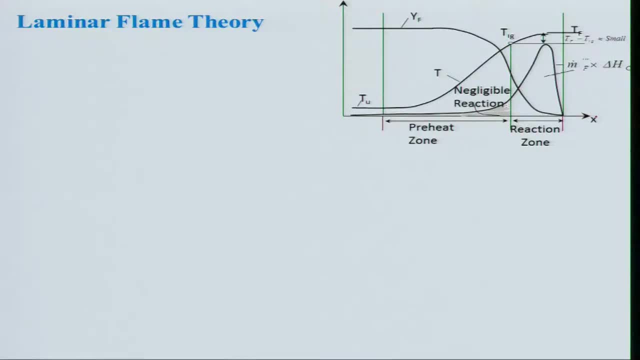 that this is our, as I told you, is the reaction, the full flame And if I look at, you know, along with x direction, when x is very far away, that means x is infinity. what will happen to temperature? because temperature profile I have shown here, temperature gradient. 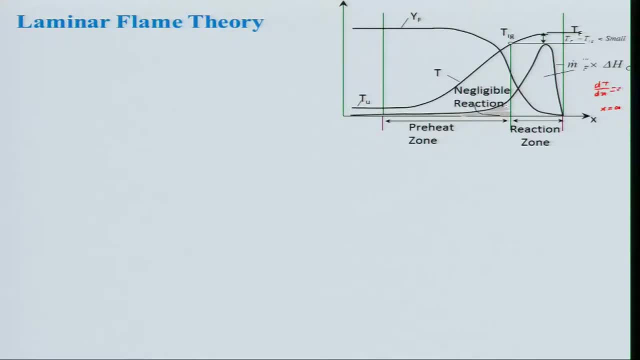 will be d, t by d, x will be 0, yes or no. and this is I am starting from here, this is my origin. So, towards, if I go towards, you know, away from the origin, towards the left hand side, This will be minus infinity. the x is equal to minus infinity. what will be the temperature? 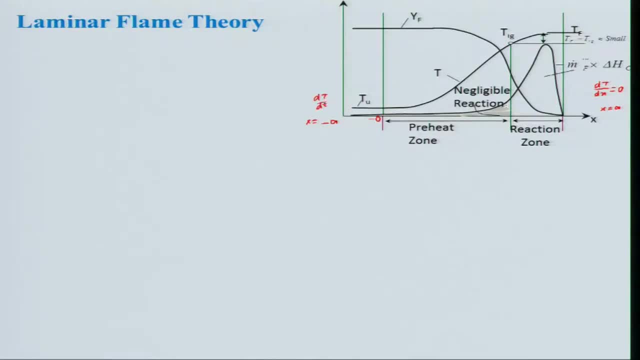 then gradient it will be again d. t by d x is 0. similarly, for mass fraction of fuel oxidizer, you know will be valid, this condition will be valid. and keep in mind that we are saying that in this reaction, this is the reaction zone where the t ignition will be, there, which 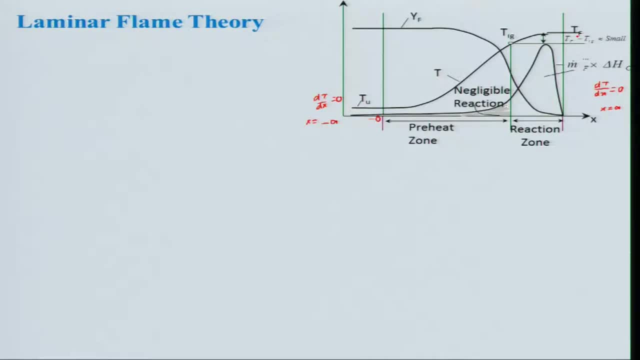 is closer to the t f. that is again an assumption we are making but it is not bad. that means t f minus t i g is very, very small. this assumption will be using for analysis, for actually deriving a relationship for burning velocity. If you look at this flame front will be moving. 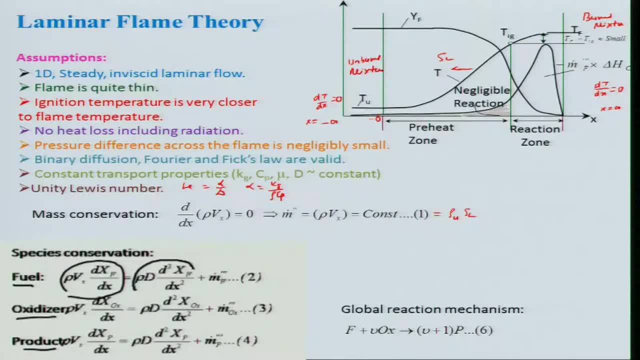 be equal to the diffusion term And the mass consumption term. consumption of fuel: mass consumption of fuel: And if you look at this diffusion term is rho- D, D square x, f divided by d- x square square. And keep in mind that this diffusivity, what we have considered, is binary in nature. 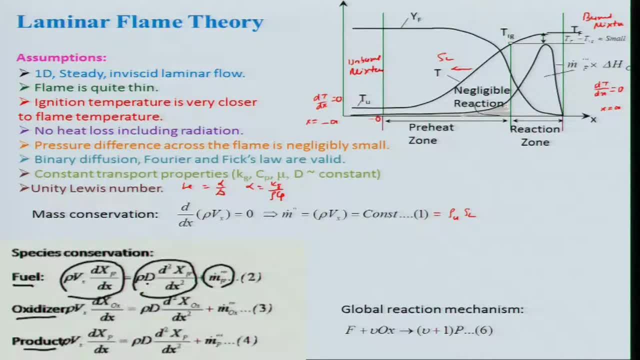 that means this diffusion between two spaces, whereas in actual system, multi component diffusion would likely to take place, And these equations will be similar for the oxidizer. for example, there will be convection term. rho, v, x, d x, o x divided by d x is equal to. 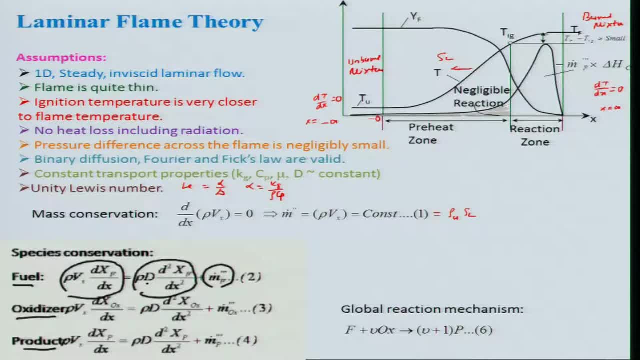 rho, d, d square, x, o, x, divided by d x square, and mass consumption of the oxidizer. And keep in mind that this is per unit volume. this mass consumption of oxidizer, even the fuel, any, everything, all this term is basically per unit volume. 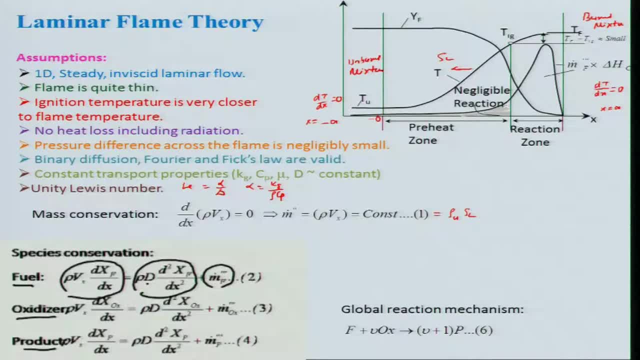 So we can get the what you call the product. that is the convection term, that is, rho v, x, d x, p divided by d x, which will be equal to the diffusion term and the mass generation of the product. The diffusion term will be rho- d d square x p divided by d x square. 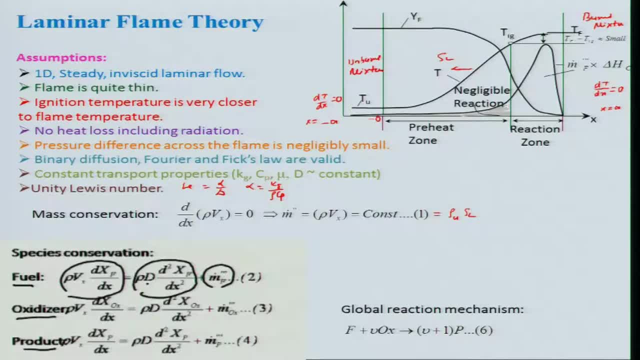 and the mass consumption of the product. we have considered as we have taken in the global kinetic, So we know the name of the explosive. that is, the one mole of fuel is reacting with new mole of oxidizer which will go in to the new plus one, what you call gram of product. So 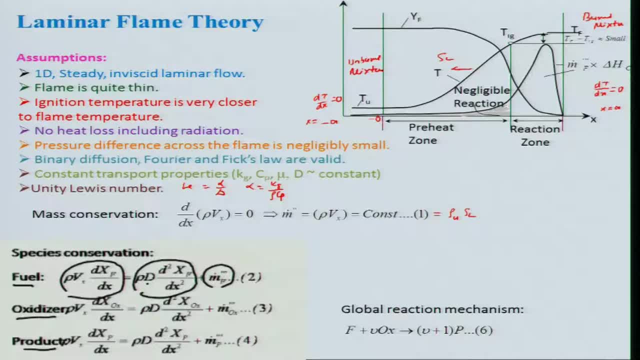 therefore, we will have to solve these equations and to get this, each mass fraction of fuel and oxidizer and product, So energy equation will be having similar form, that is, rho, v, x, d x, c, p, d t by d x, o x divided by d x square, And this is known as P? T by d x square. you. just have to add this, all the product, You get the mass fraction of fuel and oxidizer, And then the energy equation will be having similar form, that is, rho, v x, d x, to the power derivative d by d x square. So must be. this is our current general equation for energy equation. 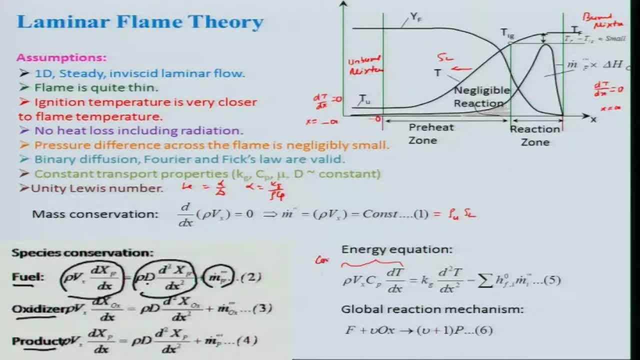 this is your what you call convection term and this is your conduction term, and this term is your what you call the heat generation or heat release right. That means H, f, i, not m, dot i f. i can be fuel- in this case, oxidizer and product. So let us look at how we can. 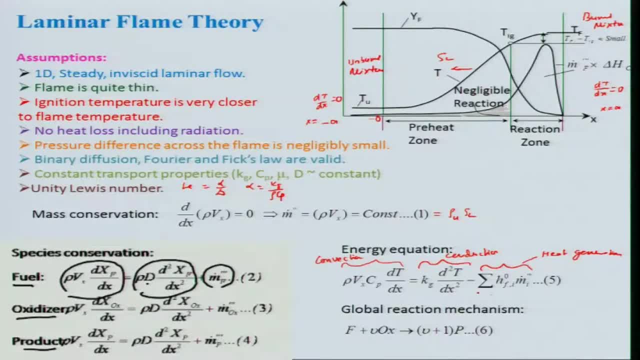 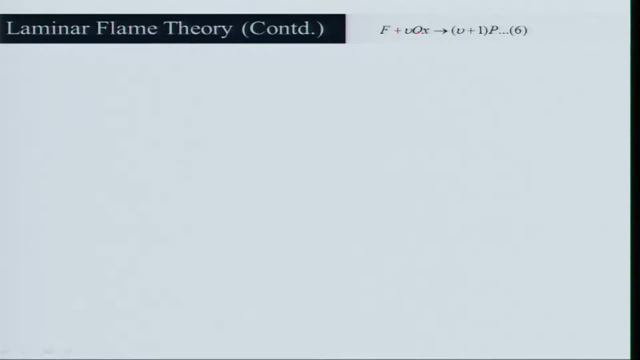 expand this term. you know and see this term particularly So if you look at- we are looking at this: 1 kg of fuel reacting with new kg of oxidizer going to the product of new plus 1 kg of product. So we can write down that m dot, triple dash f, that is the mass of the. 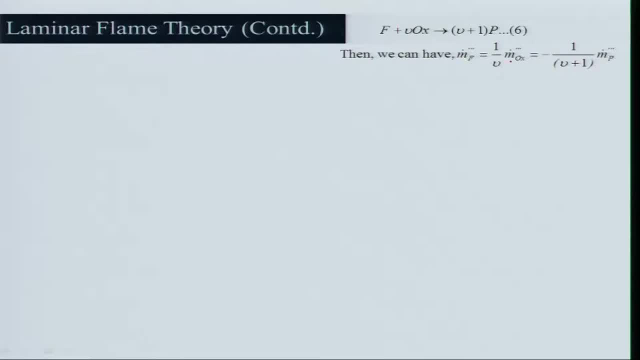 fuel per unit volume being consumed is equal to 1 over nu m dot triple dash o. x is equal to minus 1 over nu plus 1 m dot triple dash p. why minus? because this fuel and oxidizer is being consumed whereas product is being formed right. instead of writing minus here. 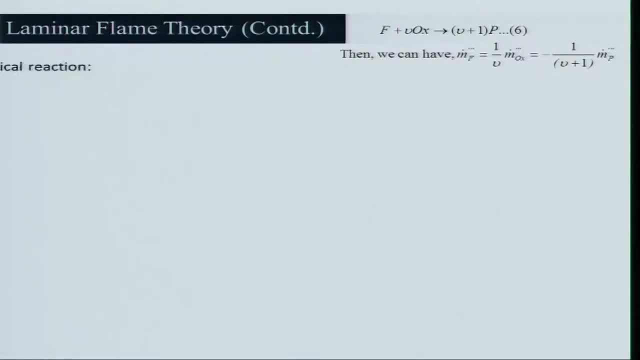 I have put here, So it is. so if I do that, like let us look at how we can do, I can expand this term H f, i, m dot i. I can write down H, f, i, H, f, f, o, plus m dot, triple dash, f right. 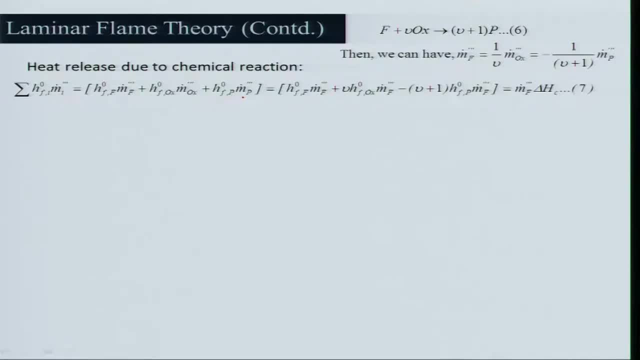 and similarly I can write down for oxidizer and for the product. If I substitute this values, you know, like for oxidizer, what it would be: m dot triple dash o. x will be nothing but your nu plus m dot triple dash f. So that is the this. 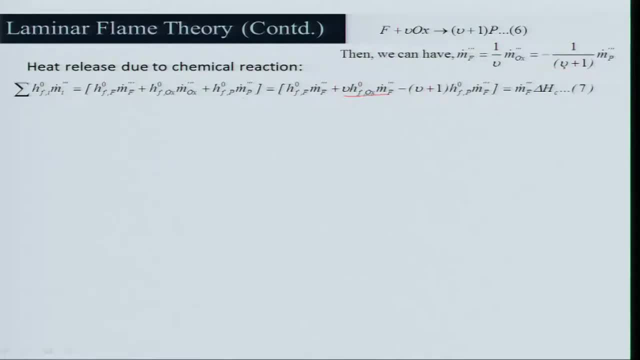 term, right. Similarly, from here I can get to the this term. if I take this m dot f out what I will get, I will get H f plus nu, H f oxidizer minus nu plus 1 H f product, and that is nothing but your heat of reaction. this is your heat of reaction, right? So what is eventually? 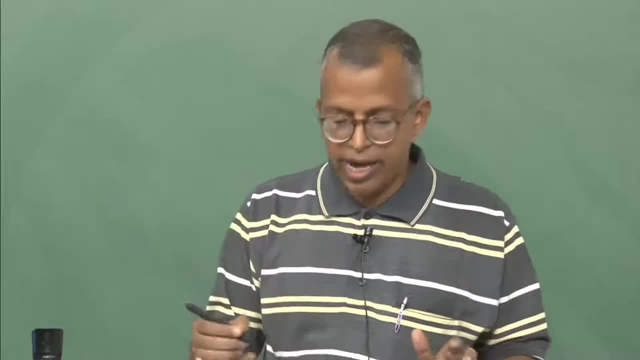 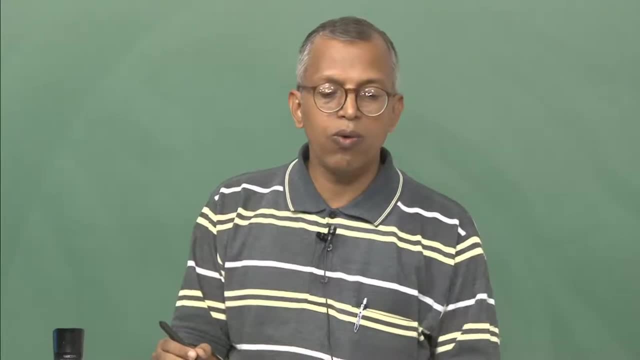 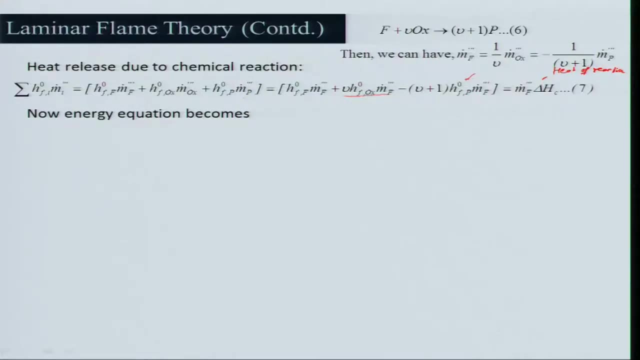 it is coming NE, That those things will 1958.. very easy to look at that. I can express in terms of that. So now what we will be using, as I told you that we will be only considering the energy equation as the Lewis number equal. 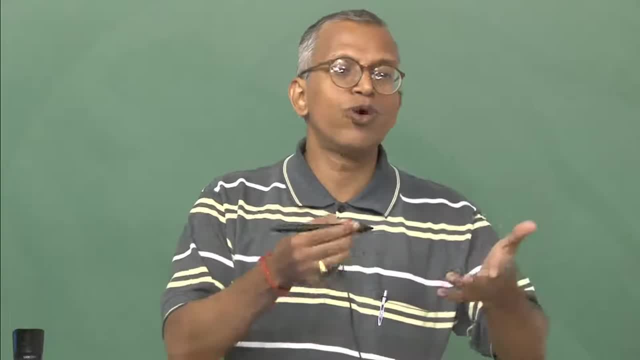 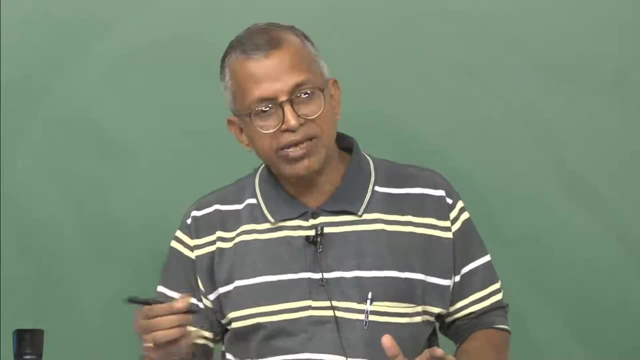 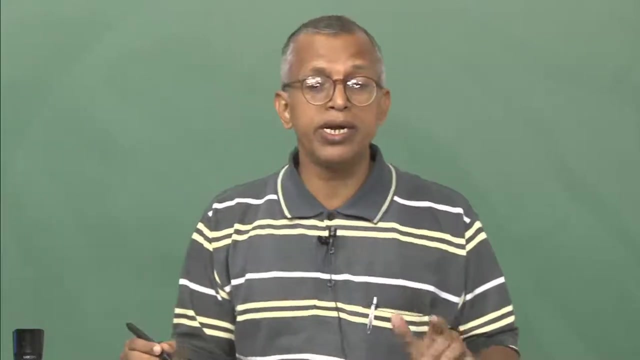 to 1.. Once we solve that, we can really look at how this fuel or the oxidized mass fraction changing with respect to the, you know, x axis or along the length of the flame. So that can be, and that is a very important assumption which we will be discussing about when we 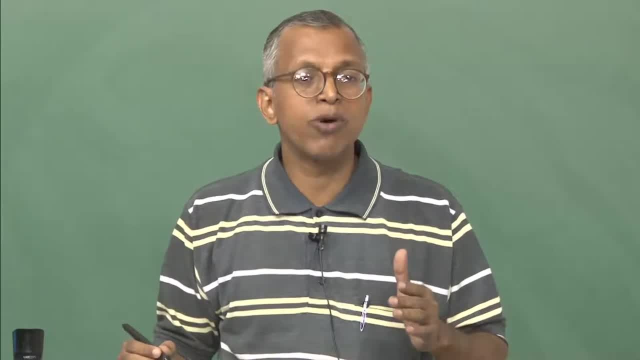 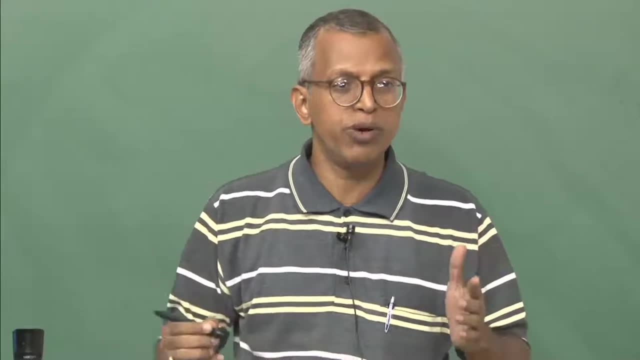 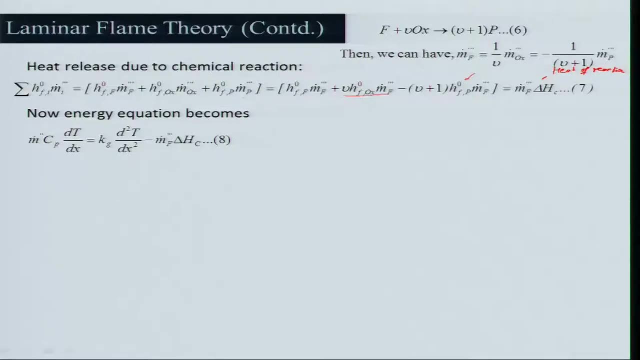 will be in detail when we are discussing about droplet combustion and that is, we will be using one known as Schwab-Chaldeau-Beach. you know transformation that we will be doing, and here I am dealing little different way, So I want to give both flavor. this is more. 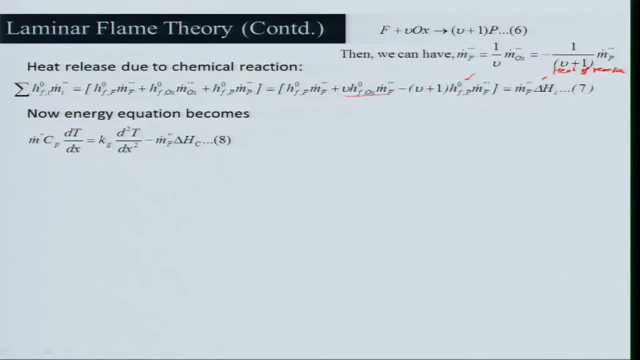 what you call Physical and that is more mathematical or mechanical. So let us look at this energy equation you know becomes m dot, C, p, d, t by d x is equal to k g d square d t by d x square minus the heat release term. What you could observe here what kind of equation it is. I 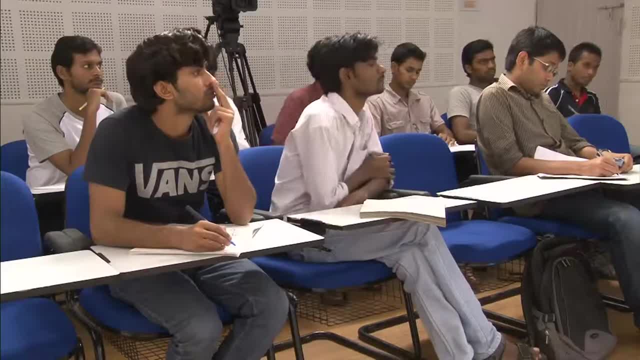 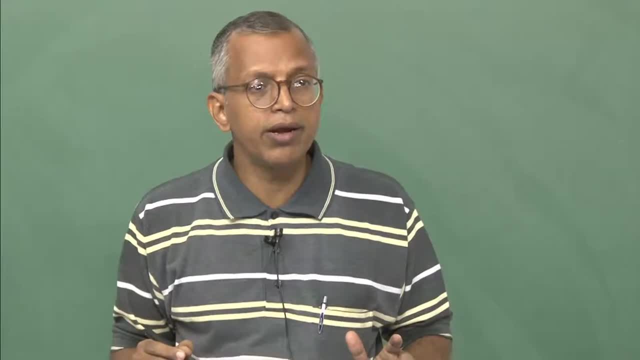 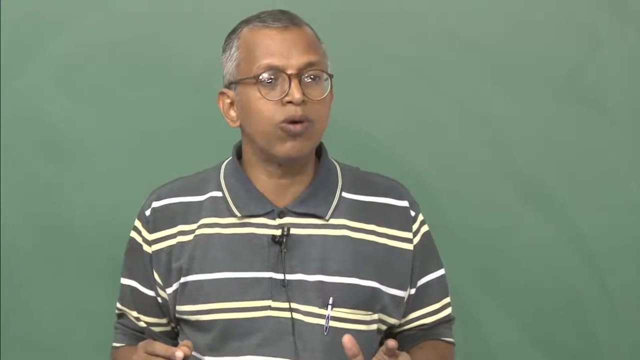 need to solve this equation 8. could you observe? is it possible? I can solve this equation. it is a second order Equation, or not? right? and it is a non linear and couple equation, right, yes or no? can you really solve? is it possible to solve with your O D? you know, you have, you have learnt. 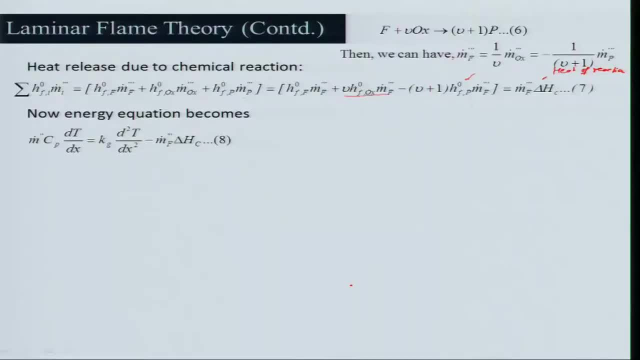 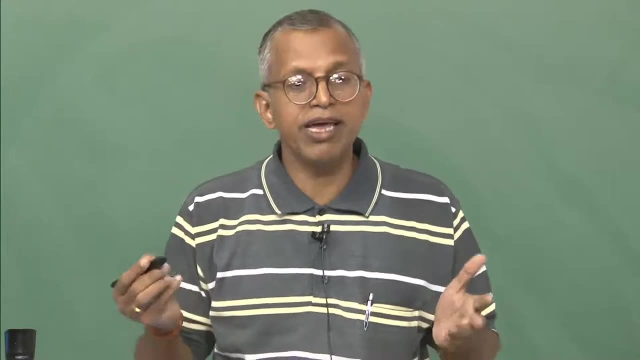 about this is a, O, D ordinary differential equation. can I really solve this equation? because if you look at m dot triple dash a f, right how it will be. Look at Arrhenius form of equation That is m dot triple dash a f. if i look at on global kinetics, you know it will be a f. 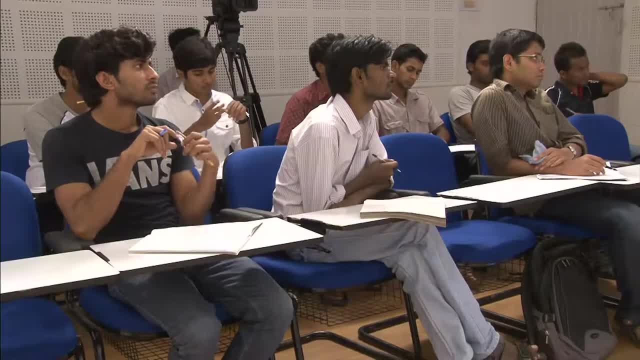 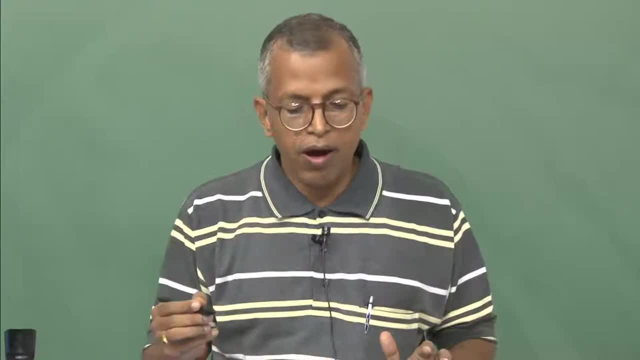 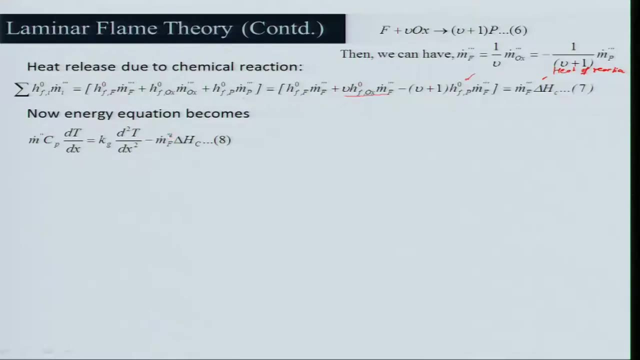 then C, f, concentration of F. of course you will have to in terms of mass fraction. if want to put it will be talk in terms of molecular weight multiplied into C of oxidizer, E, power, T, E by r, T, right? So if you look at this term is a very, very non. 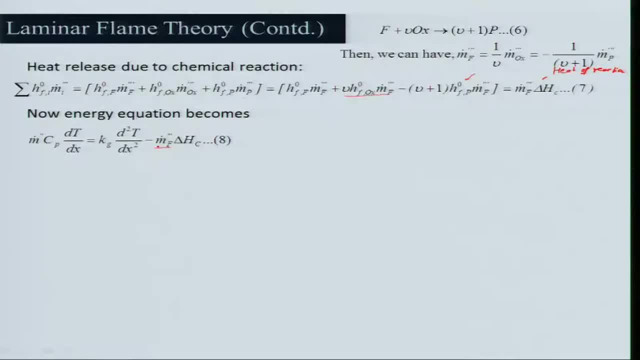 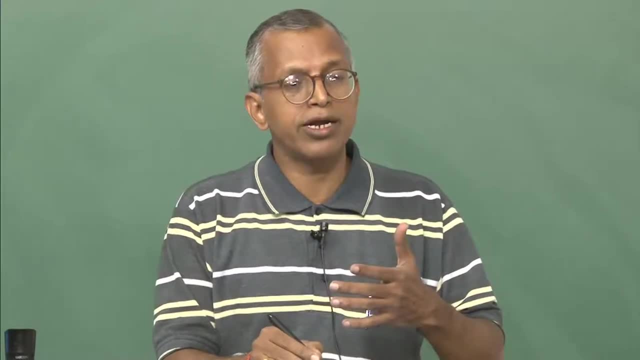 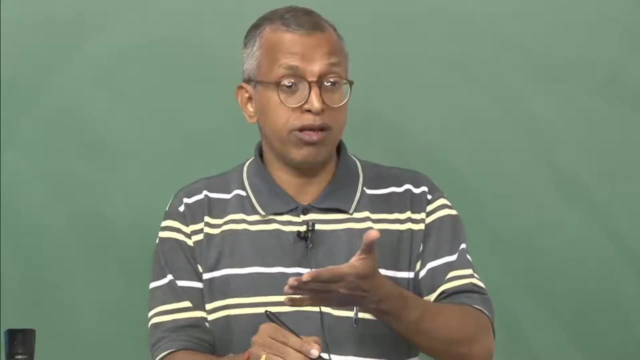 term, because I should know the temperature, I should know the activation energy, I should know the pre exponential factors And those activation energy pre exponential factors will be dependent on what is the full air ratio you are talking about and also it will be dependent on temperature, very highly. temperature, you know, because e power to the, you know e. 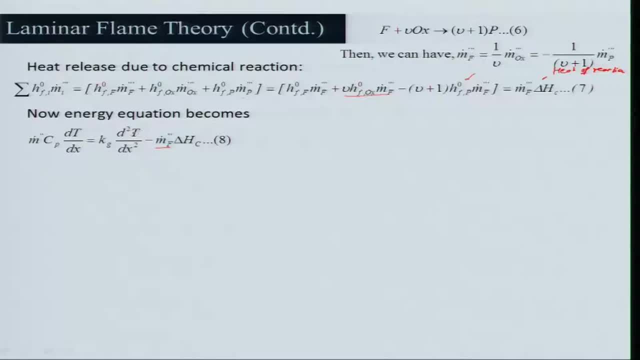 minus r by r? u t. So therefore it is: you do not know temperature. therefore you are solving this equation. therefore it is quite difficult do that. So how to go about we will see. we will go back to this diagram. if you look at what we, 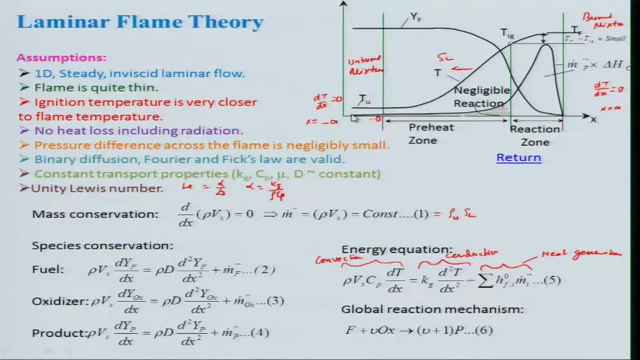 are doing, I mean basically what we will be doing to solve this equation, because it is a quite complex non-linear- And what we will be doing we will be basically looking at in the these zone, in the preheat zone, which is more predominant. here there will be convection. 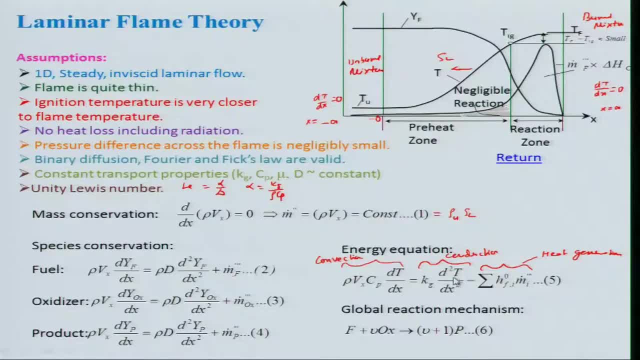 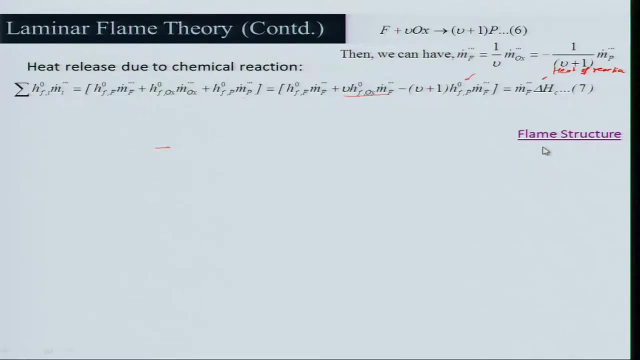 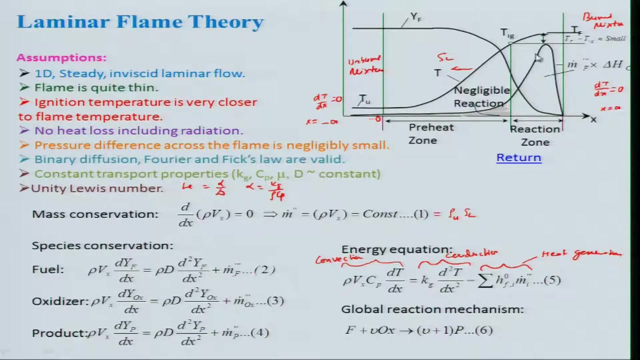 and if you look at this equation, convection and conduction. But, however, the heat release term will be negligibly small because this is a very small portion. that will be very small portion. this is very small portion, So we can neglect that. and in some zone, what? 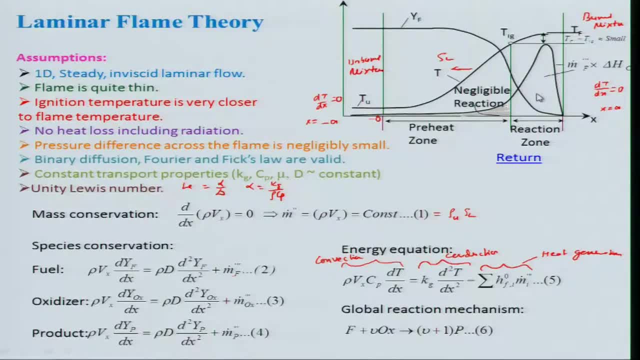 we will be doing. we will be basically looking at in these zone, in the reaction zone, Where we will be neglecting the convection. that means whatever heat will be released will be carried away by the conduction because the temperature gradient is very high. So 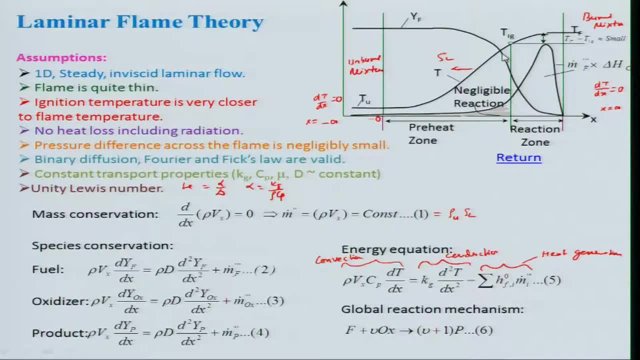 the gradient is very high, So therefore we can neglect that term. So that is the way which will be looking at it, and I have already told you that this is your. what you call at x is equal to minus d, t by d x 0, and x is a positive infinity. therefore, away d. 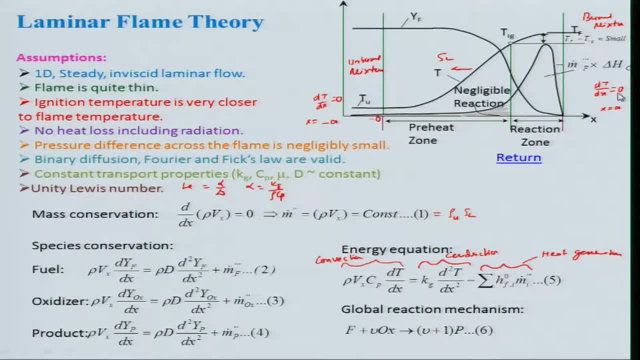 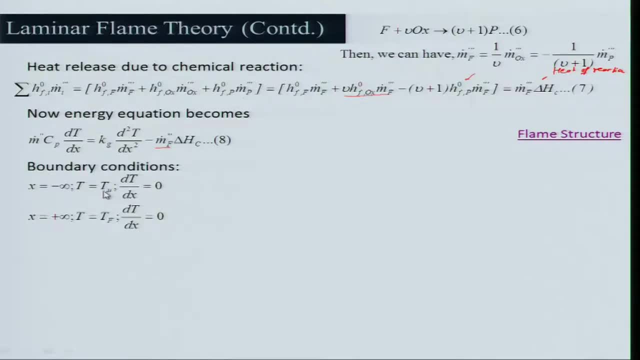 t by d x 0 is a very away from that. So, and what are the boundary condition? if you look at- of course I have already talked about it- t is equal to t u x minus infinity d. t by d x 0 x positive. 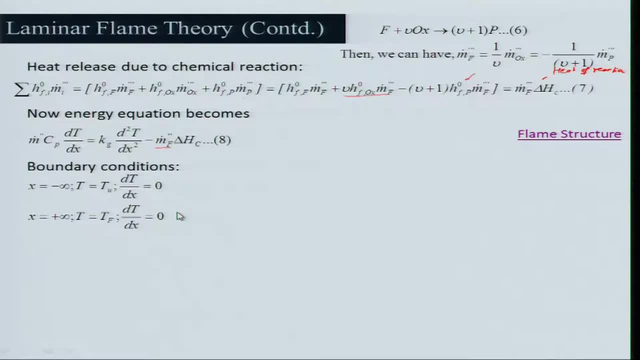 infinity it will be. t is equal to t, f, d, t by d x 0.. And, as I told you, we will be looking at this preheat zone. in the case of preheat zone, this will be 0. in this case, this will be 0.. 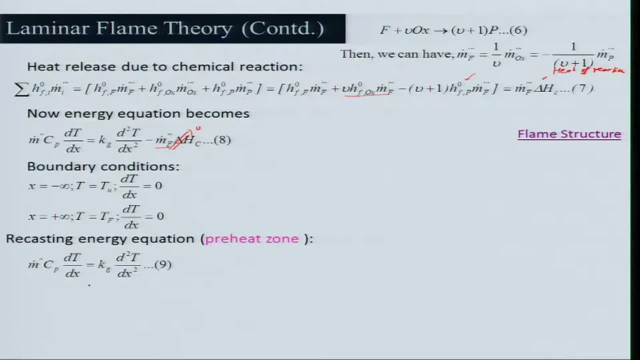 In the preheat zone. for preheat zone, this will be 0. therefore, you will get m dot c, p d t by d x, k, g d t square by d t x. that means the whatever you know, the conducted, you know like heat is coming from the reaction zone. it is being, you know, balance between the conduction. 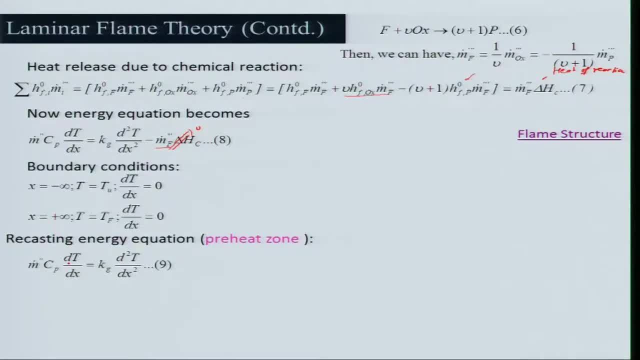 and convection through conduction is coming and it is convected away. that is the balance, So it. and if you look at for the Preheat zone, the, of course these are the condition has to be value. that is of course at the x will minus infinity. t is equal to t u d t by d x 0, x is equal to minus x ignition. 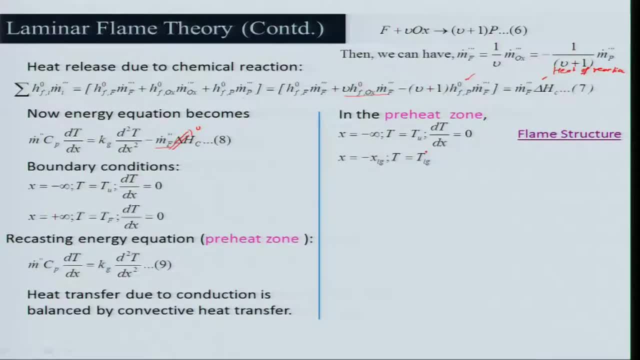 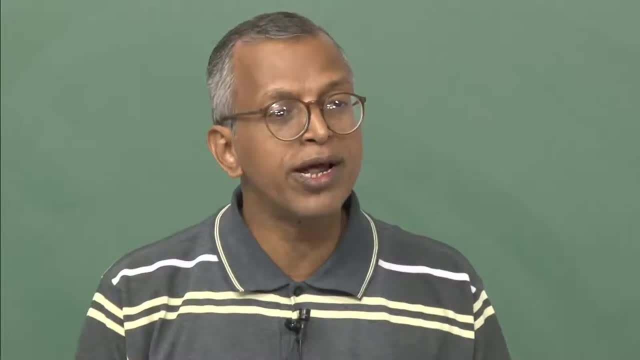 you know that I have showed you at that point. t is equal to t ignition. See, basically, you want to decouple- you know this equation- and solve, divide and rule, basically. but you are landing in one problem. I do not know this t ignition, I do not know, you know. 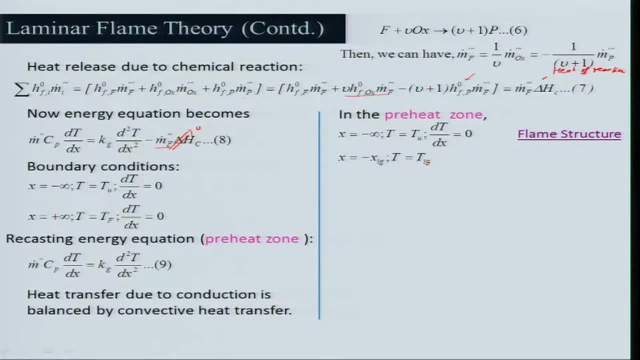 you are trying to solve, but you are landing in problem. So how to do that we will see little later on. So if I- what you call- integrate this equation, what I will get d t by d x ignition is equal to m, dot, c, p, k, g, t, i g minus t u. 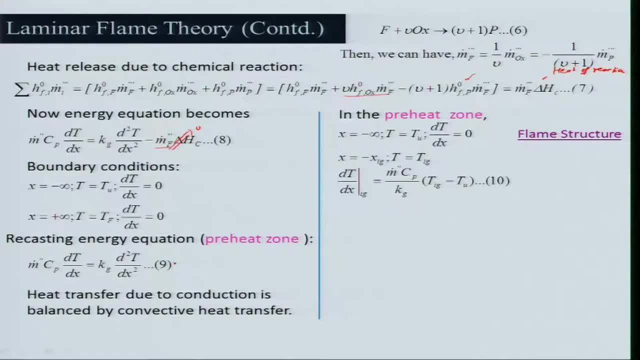 I am just integrating this equation by integrating equation nine, by integrating equation nine, So we can get d t by d x, because the other term, it is 0.. So that is going away, and then you are getting m, dot, c, p, k, g, t ignition minus t u. So in the reaction zone, however, what? 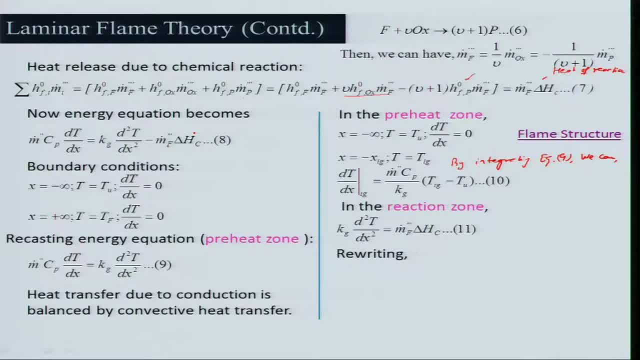 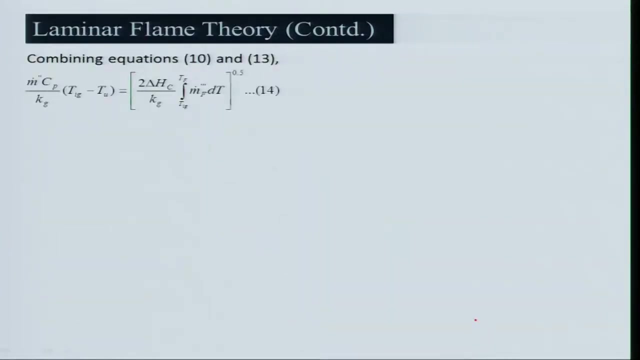 will happen in the reaction zone. what we will be doing, we will be basically looking at this. convection term will be negligibly small, only the conduction. So we are avoiding this gradient, temperature gradient at ignition point. So that is the way we are doing. So, combining this equation ten and thirteen, we are getting m dot double. 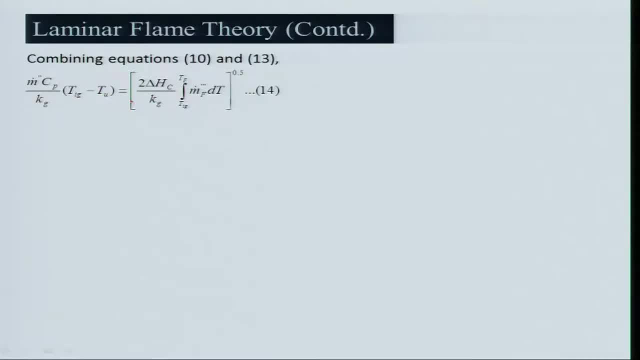 dash c p by k g, t i g minus t u equal to root over 2 a delta s c, k g integrated over m dot triple f d t. it is integrated over t ignition to t f. So if you look at, still we are not solving because we need to integrate this, you know. 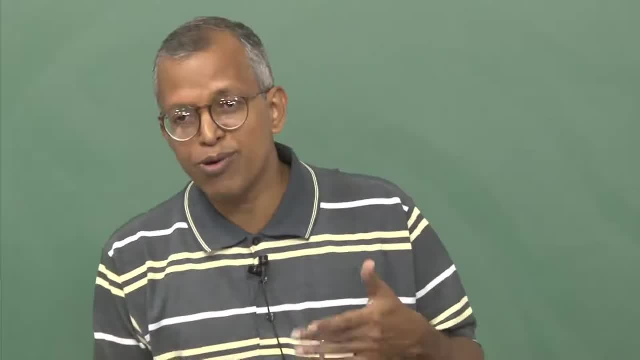 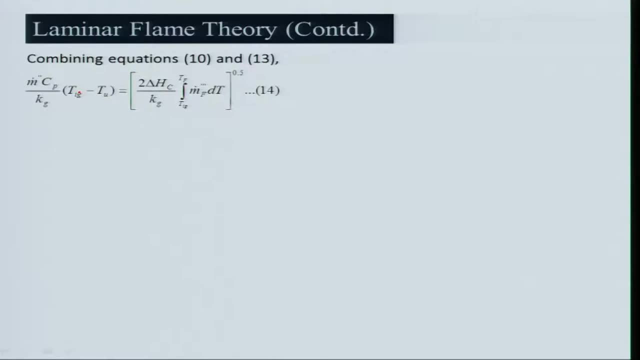 integration. that is not really possible because you do not know that temperature, how it is varying with temperature right and the t ignition is also not known. So you will have to do some approximation for that and of course I can simplify this: m dot dash is equal to. 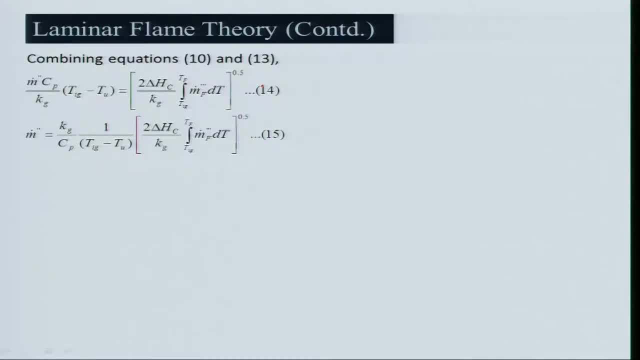 k g by rho c p 1 over this, Just rewriting this equation fourteen in this fashion, nothing more than that. So we know that m dot triple double dash is nothing but rho u s l from the continuity equation. So I can write down over here, you know I can. 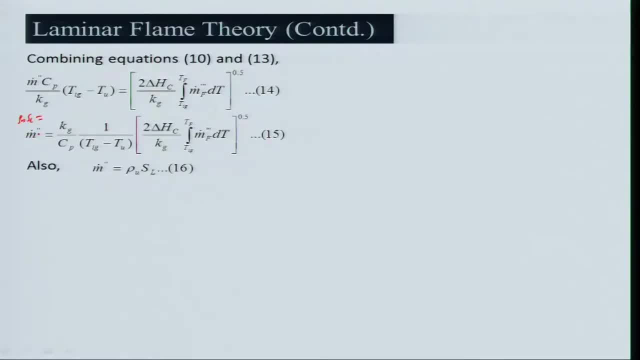 write down rho u, s l is equal to this. So then I can really look at combining this equation fifteen and sixteen. I can get s. l is equal to k g by rho u c p, because rho u has gone over here. So rest of the things is same as that of the equation fifteen. right Now, what we need: 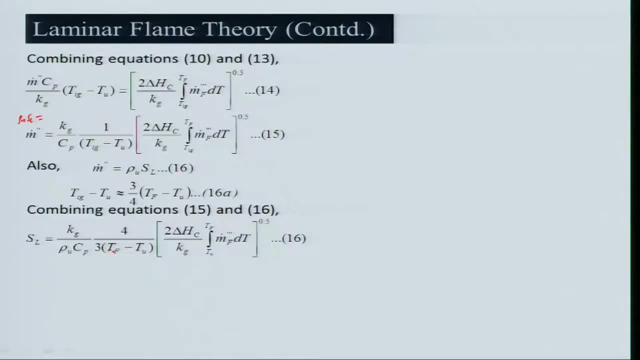 to know, but still you know that you know. here I have introduced t f minus t? u in place of t ignition and t? u. right What we are, assuming that t ignition minus t? u is approximately three by four of t f minus t? u. right, If you look at what I am doing? right? this is my t. 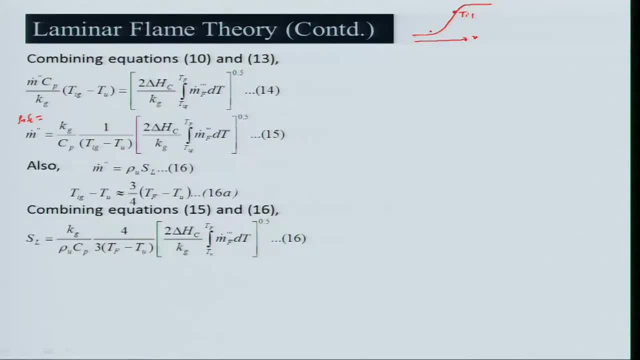 ignition this x direction. this is your t? u and t f. What I am saying? t ignition minus t? u right. this portion is nothing but three fourth of t f minus t? u right, and that is a fair enough to say that. but this is a adhoc. there is nothing sacrosanct about it, but 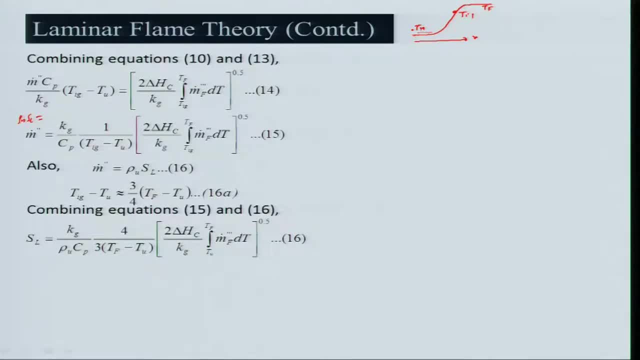 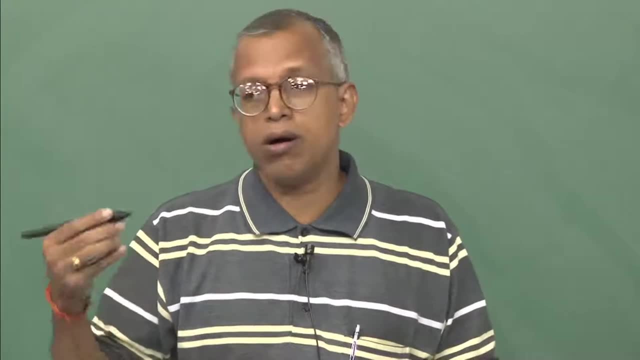 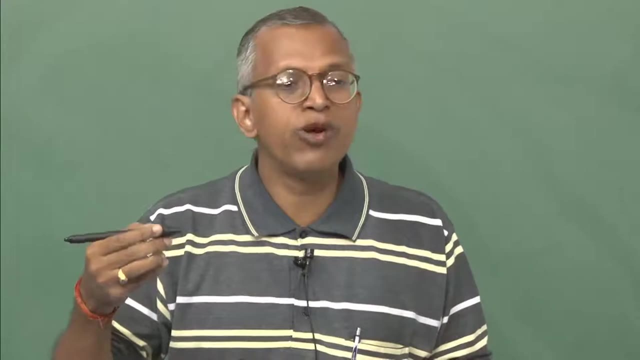 we are looking at flame temperature profile from experiment and approximating it and doing that right. So it may be valid for you know, limit mixtures. it may be valid for the what you call stoichiometric, where the reaction will be governed by the activation energy, right. So therefore there. 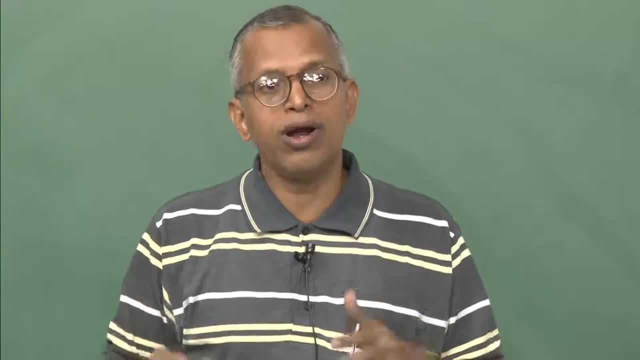 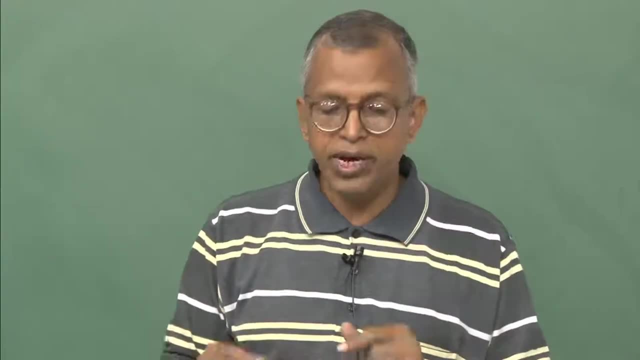 it will be valid, whereas for the limit mixture it cannot hold good. nor even for hydrogen air, where the activation energy is very, very small, you know, it would not be valid. So this is the limitation of this kind of analysis. So then, a still, we are assuming that this. 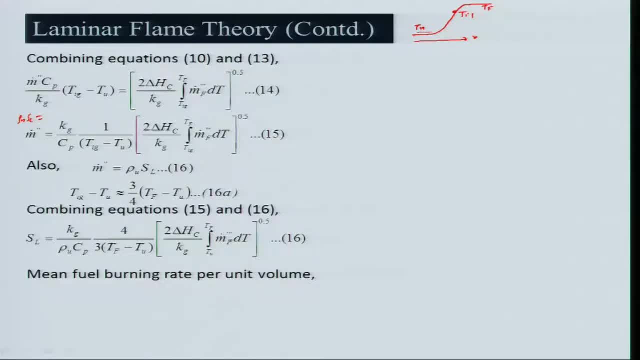 is a adhoc. So we are having a problem with this m dot triple dash f d t by t f. but we can assume that mean fuel burning rate per unit volume will be. you know, m dot f triple dash, that means this term. I am saying that is nothing but m dot f triple dash average over the region. 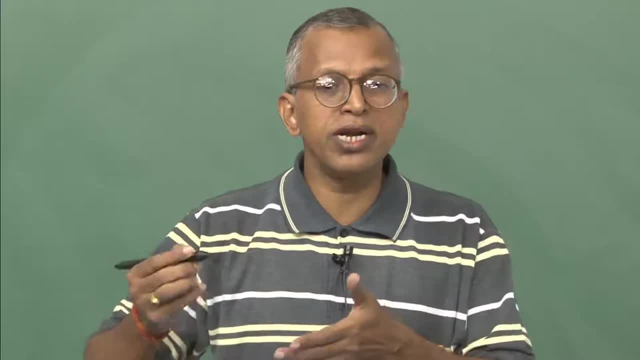 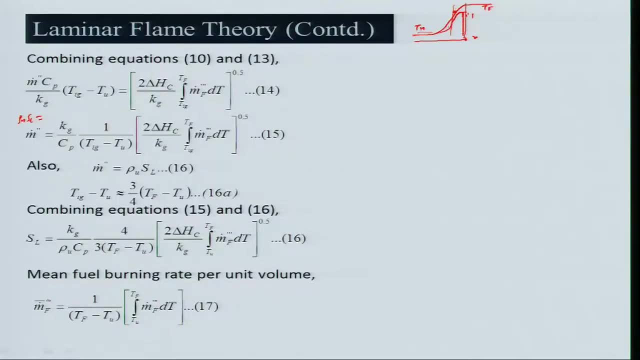 what is happening? Because it is changing. you know, this mass burning is changing in the region, from here to here. if you look at this zone, it is changing. This is, like you know, coming over here. this is your m dot f right. it is changing reaction. 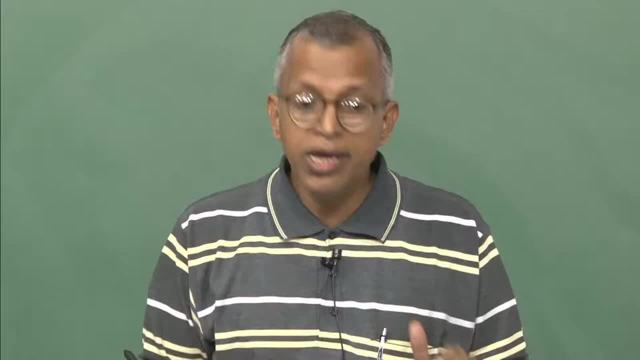 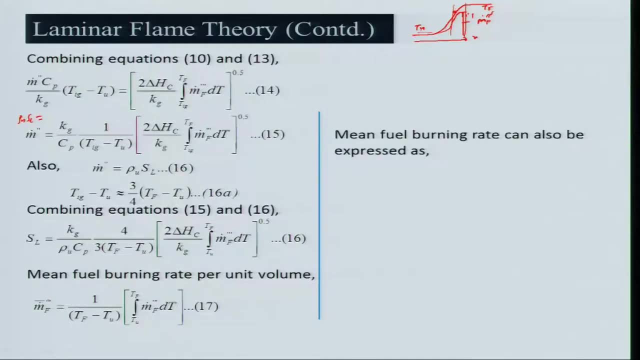 rate, in other words, right. but here we are saying no, no, we are not bother about integration, we will say it is average. what is that average that will be approximated as the what you call a reaction rate, arrhenius form of reaction rate, right? What is that? molecular weight? 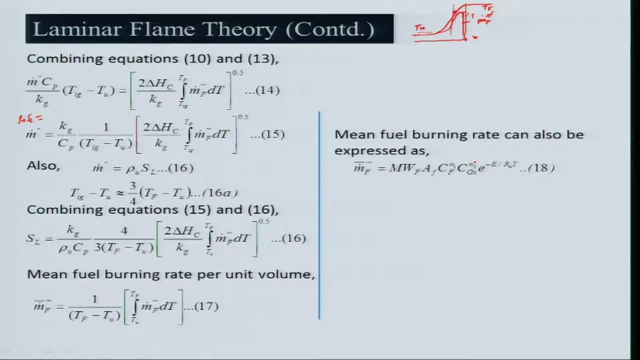 of the fuel: a, f, c, f, n, 1, c, oxygen, n, 2, e, power to the e by r u, t And, if I know this, values a, f, e and then concentration of that which will come from the where. what is the fuel air ratio? I can estimate this thing right, provided I know this temperature right And 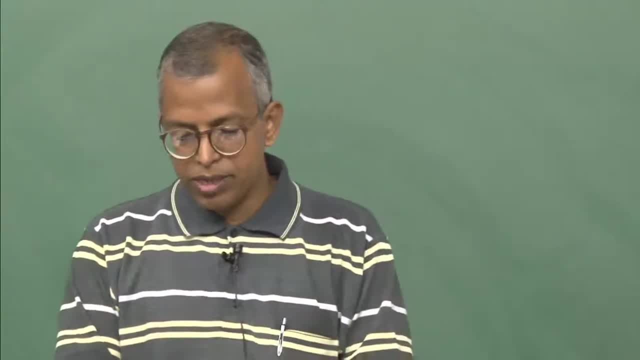 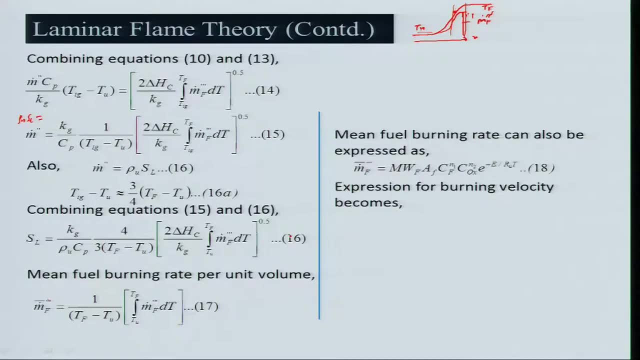 that temperature will be doing some average one kind of things right. So expression for burning velocity: That means that is the equation c sixteen becomes what, like you will look at what I will do. I am taking this kg by row c, p inside, So therefore it will be square inside of. 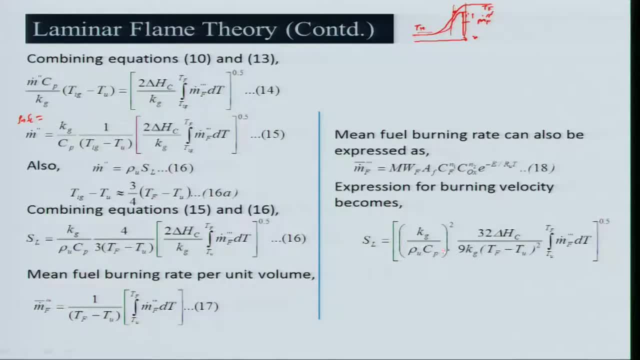 square root. point five is nothing but square root, and then I am taking also four and three, so four, four, it is sixteen. sixteen root, two, thirty two And three: square is nine. I have taken inside nine. k, g is already there and T f minus T u whole square, because this term I am taking inside. 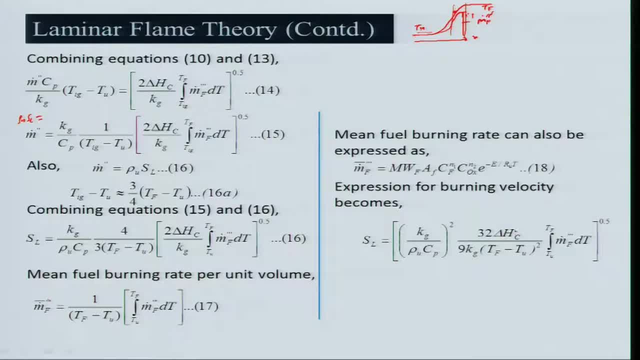 the square root. So it will be square, but we can you know like look at this delta S c and whether we can express in terms of temperature that can be approximated, as delta S c is approximated, nu plus 1 C, p, T, f minus T u. So what we will be doing instead of this, I will be writing. 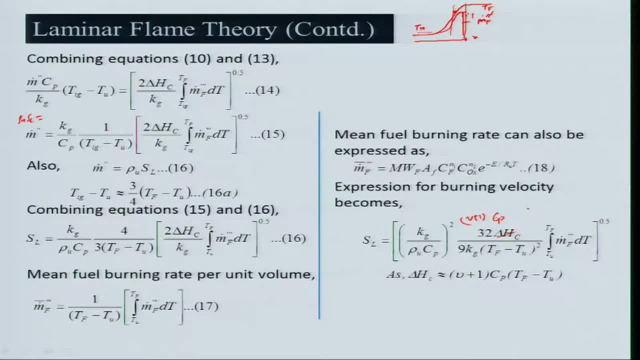 down C p nu plus 1 T f, minus T u in place of this. So what will happen then? this T f will be cancel it out, the only one T f will be there, and this portion, this what it would be. this will be: m dot triple dash, f average. this equation, yes or no? 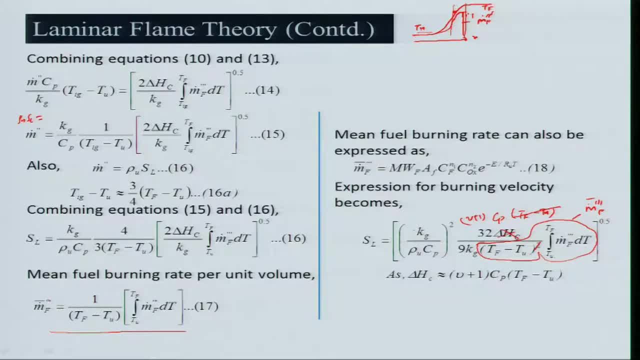 So I, and if you look at what is this one kg by rho C p, that is nothing but alpha thermal diffusivity. and if you look at kg and there is a C p, So if I look at what is alpha, Alpha is nothing but kg by rho u C p. So C p by kg will be. you know, if you look at this, 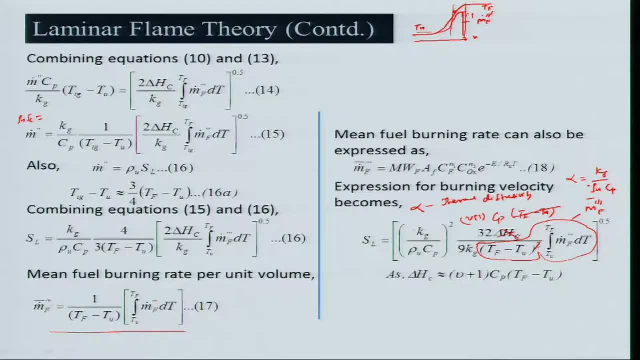 is alpha square alpha. I can write down basically this: k g will be alpha rho u c p. So in place of this, I can write down as alpha rho u c p: this c? p will cancel it out, that this rho, because this is a rho basically. So this will be cancelling it out and rho u will be. 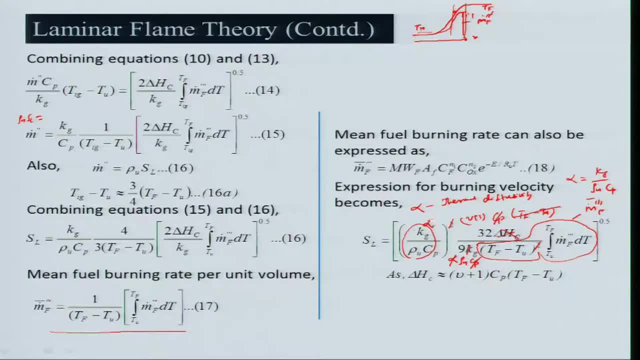 there, because this is nothing but your what alpha, square alpha. So therefore I will get S. l is equal to 32 alpha divided by 9 rho u nu plus 1 m dot f, triple dash. this is a very elegant, you know expression, But if you look at how many approximation we have, 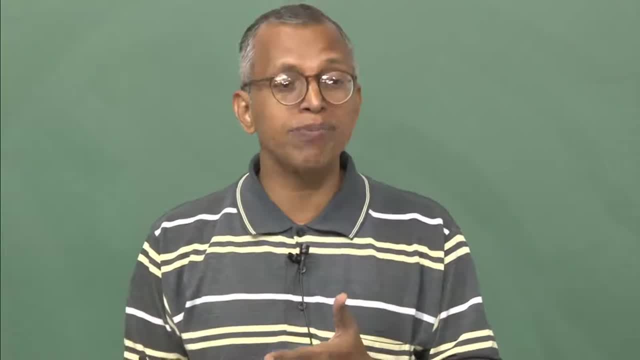 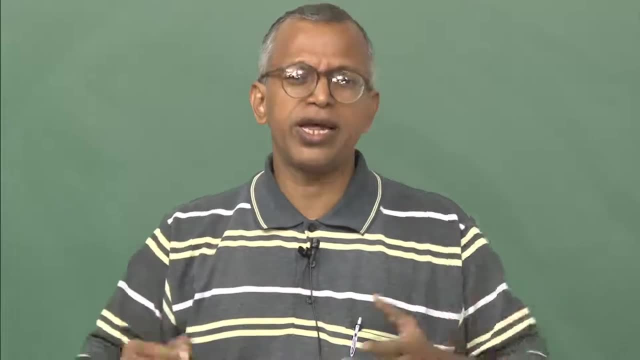 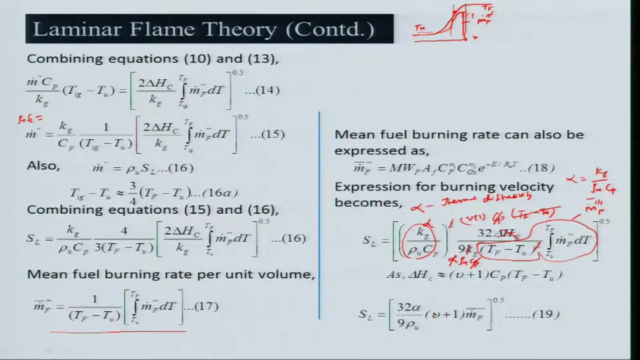 done and what is the sanctity of those approximation one has to worry about. but however, we are getting a close form solution And that is we can see. So from these what you can see, that burning velocity will be dependent on the nu. that means fuel air ratio. nu is a stoichiometric ratio in our equation.